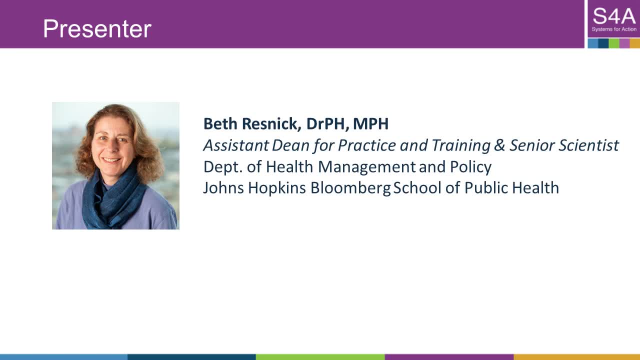 Beth Resnick, Principal Investigator, is a senior scientist at the Johns Hopkins Bloomberg School of Public Health and Director of the Office of Public Health Practice and Training. Dr Resnick was a 2012 Johns Hopkins Student Outreach Resource Center Service Learning Faculty Fellow. 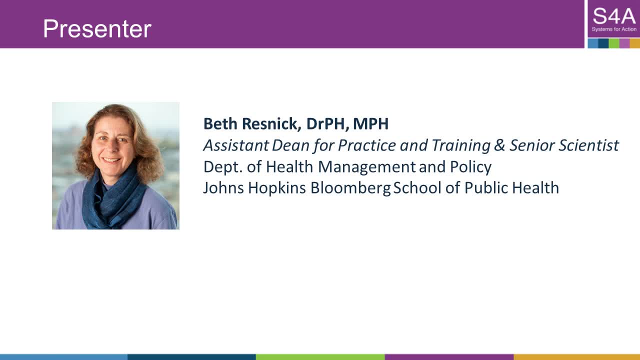 where she engaged with the Baltimore community in nursing and medical schools. She has worked with multiple faculty to engage students with communities to advance the culture of health. Prior to joining the Johns Hopkins faculty, Dr Resnick was Director of the Office of Environmental Health at the National Association of County and City Health Officials. 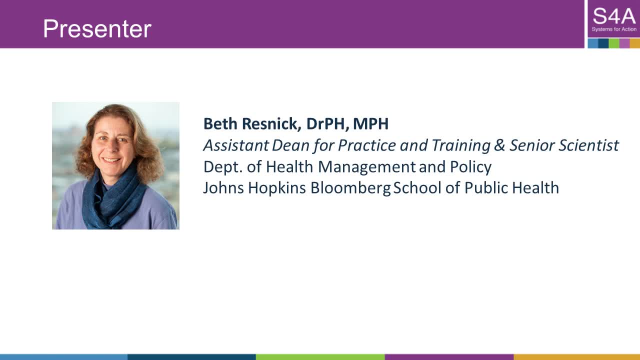 Dr Resnick was the Principal Investigator on the Development of the State Health Expenditures Data Set. David Beschey is Professor at the Johns Hopkins Bloomberg School of Public Health and directs the School of Public Health. Thank you. The Beijing University Health Council Annual buluniko. 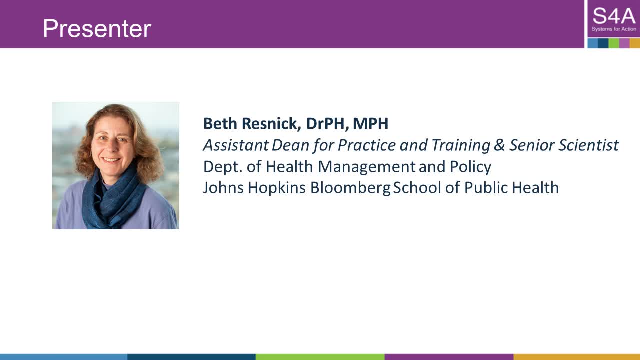 Nate Jerry two roles in the project. he will lead the proposed econometric analysis and identification of funding in equities by income level, race and county health rankings. Dr Beschey has conducted a series of analysis of state and county health spending data and work supported by theDE homage Foundation that provide a methodological. 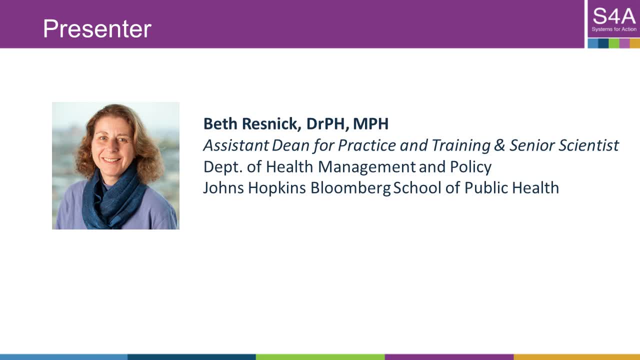 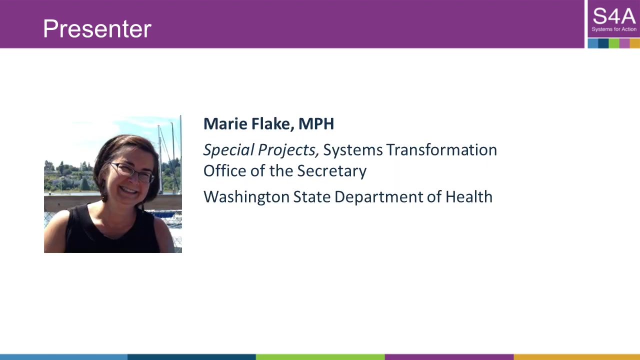 foundation for the proposed sector auto regression analysis, state and local governmental spending on medical, public health and social service spending. He maintains board certifications in internal medicine and pediatrics, as well as part-time practice four days per month at the University of Maryland St Joseph Medical Center. 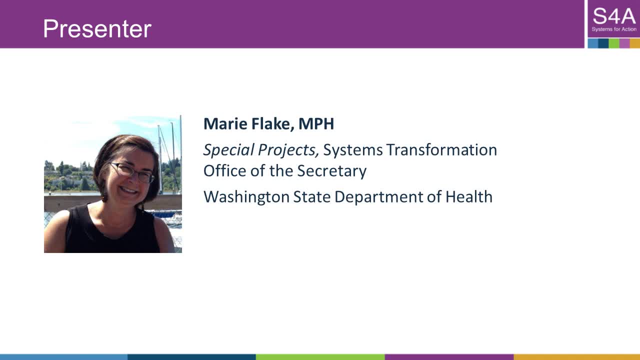 And our commentary speaker is Marie Flake, who works at the Washington State Department on the Systems Transformation Team, where her focus is on collaborative statewide effort to transform the governmental public health system. This includes further developing a comprehensive framework for foundational public health services that includes definitions of the foundation public health services, clarification of funding. 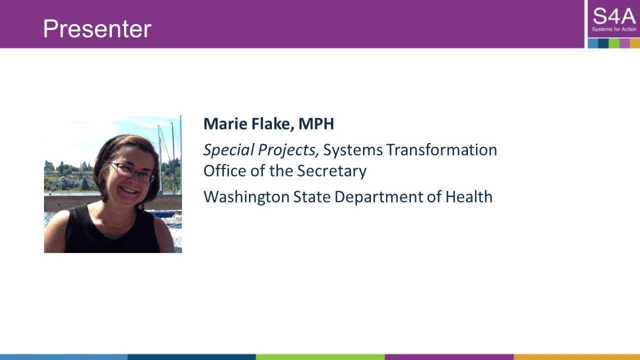 roles, cost estimates, new service delivery models, an accountability system, funding allocation, processes for routine updates, and policy and legislative issues. Previously, Marie served as the agency's liaison to the 35 local health systems and facilitated Washington's Public Health Improvement Partnership, which produced leading work on. 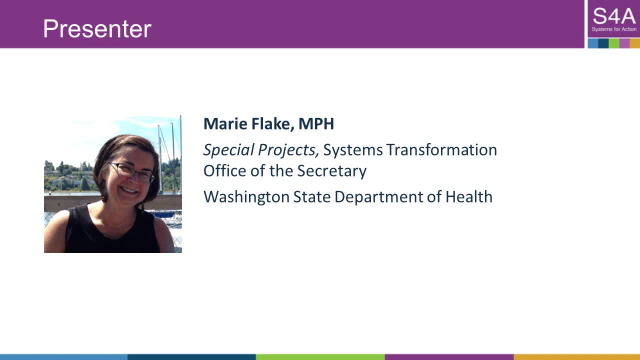 system-wide standards, system-wide performance measures and public health indicators and finance studies for the public health system. She has experience working at two local health departments in Washington State for the local public health association in Maryland, on the faculty at the John Hopkins School of. 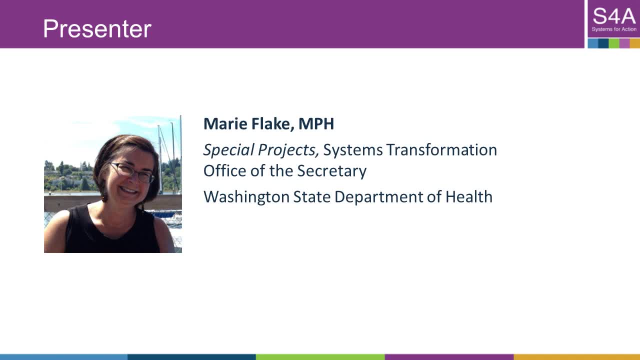 Public Health and as a registered nurse in a variety of clinical roles. And next we have Marie Flake, who is the Director of Public Health and Health Services at the University of Maryland. And now I would like to hand the program over to Drs Resnick and Bishai. 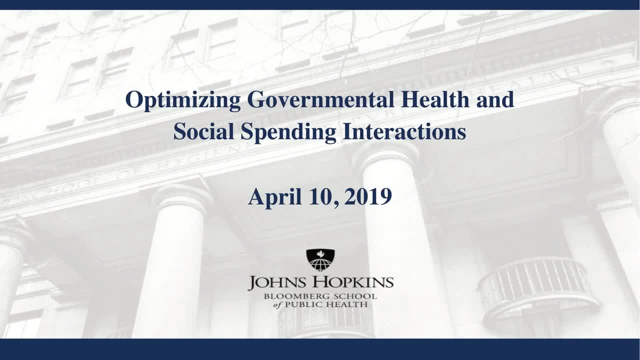 Great Thanks. This is Beth Resnick and just wanted to make sure if someone had said they had an audio problem. If people can hear, I'm assuming we're good, But if there's any problem, you guys let me know. 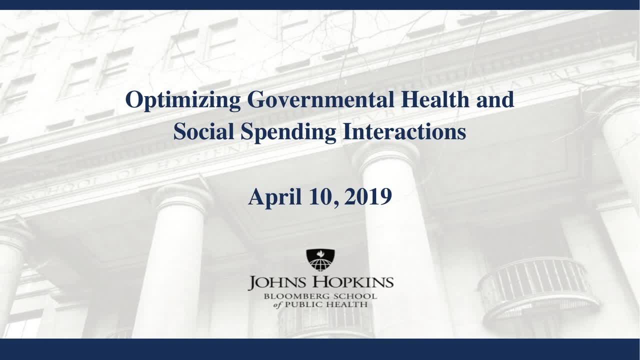 So thank you for the opportunity to share our work today. We're excited to present what we've been working on on our Optimizing Government Health and Social Spending Initiative. We're excited to share the work that the organization is doing and we're excited to 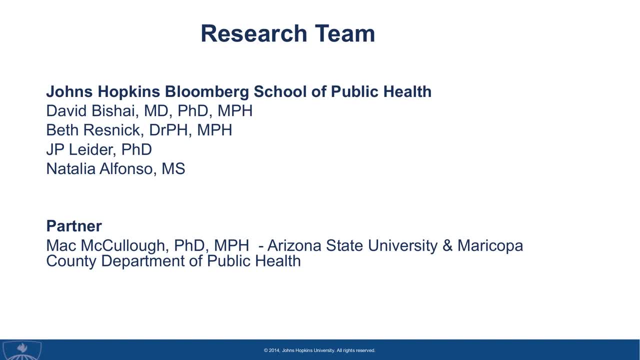 share the work that we're doing as well, So I think that's going to be a great opportunity to share what we've been working on. So this is our first public health team. We have two of our partners. This is the public health team. 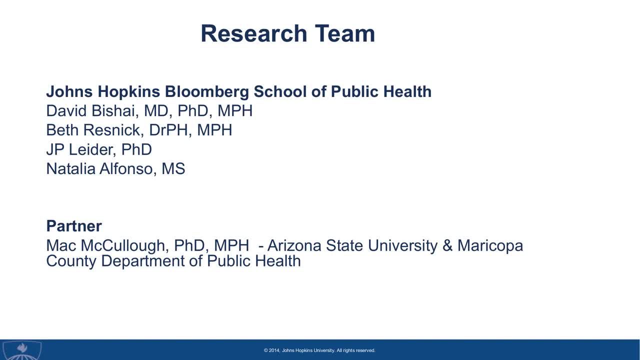 They're going to be working on the public health initiative, but we're also going to have a partnership with the University of Arizona, and they're going to have a partnership with the Arizona State University. So with that, I'm going to jump right in. 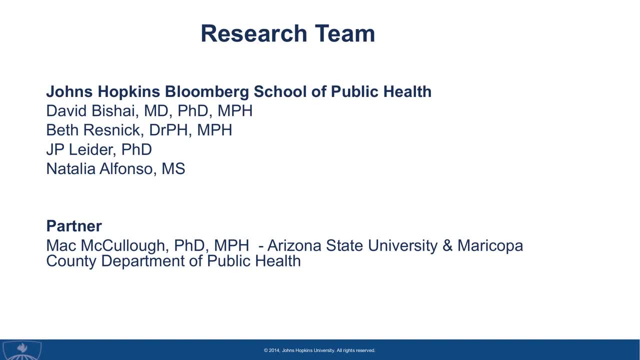 This is our research team from Johns Hopkins School of Public Health listed here, as well as our partner with Dr McCullough, who's at the Arizona State University and also at the Maricopa County Department of Public Health, And I also want to thank Marie Flake for joining us today, as it will be great to hear from. 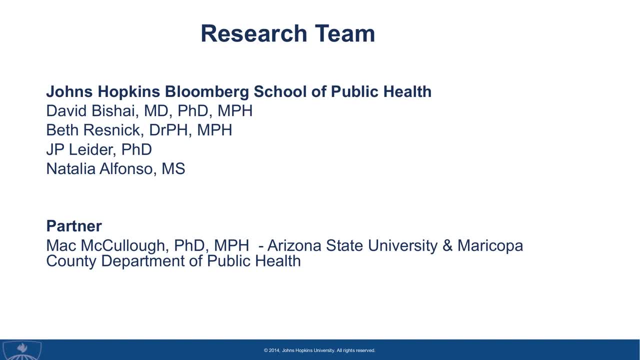 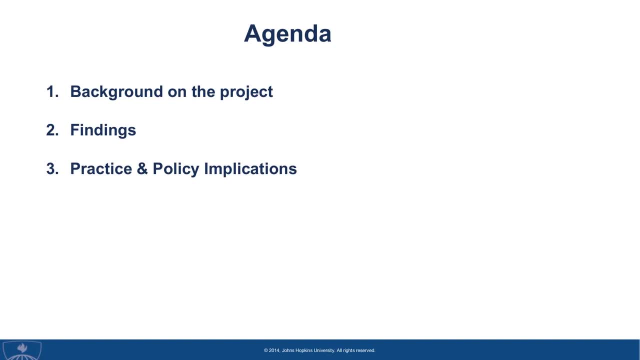 on their state level so people can really think about how they can apply this work in their own states and localities. So thank you, Marie. So, for our agenda for today, I'm going to give you a brief background on the project. Then Dr Bishai is going to be giving more details on some of our analysis on the different 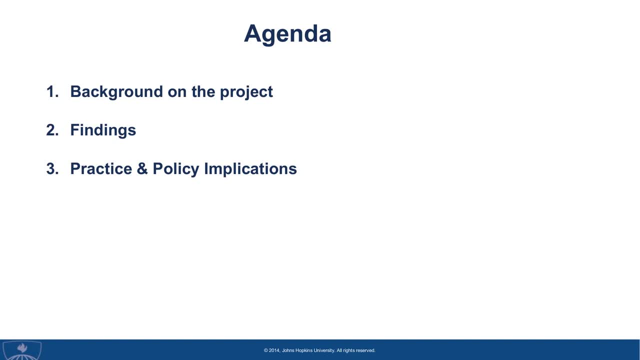 spending amounts And then we'll hear from Marie about what they're doing in Washington State. So I think our piece is more macro, where we're looking at national level spending and spending by states across the country and localities, And then Marie will give us more perspective from on the ground within Washington State. 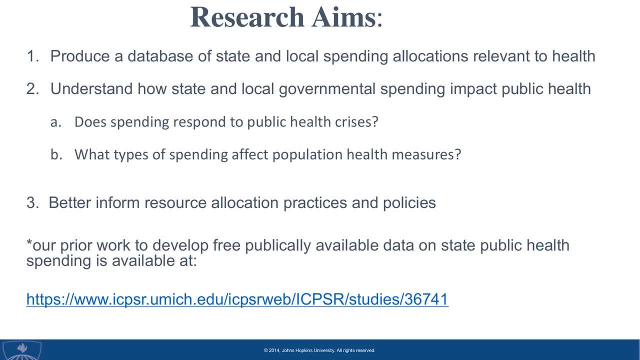 with some of the great work that they've been doing. So with that I'm going to jump in. The aims of our overall research project that we have been working on for the last several years is to really think more clearly about what we're actually spending, both at the state. 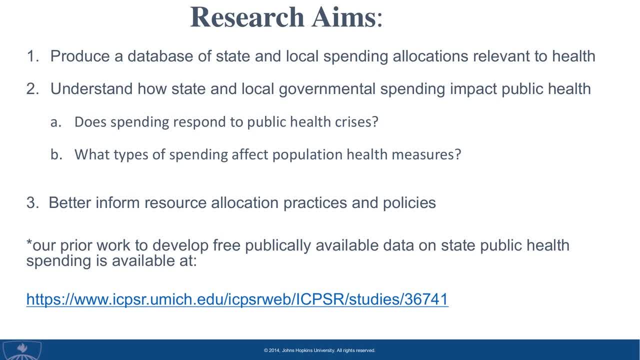 and local level That is relevant to health. And then number two here is to then think about that spending in terms of how it impacts public health, And specifically what Dr Bishai will be talking about more is: does our spending patterns respond to different public health crises and what the impact of spending overall is on population. 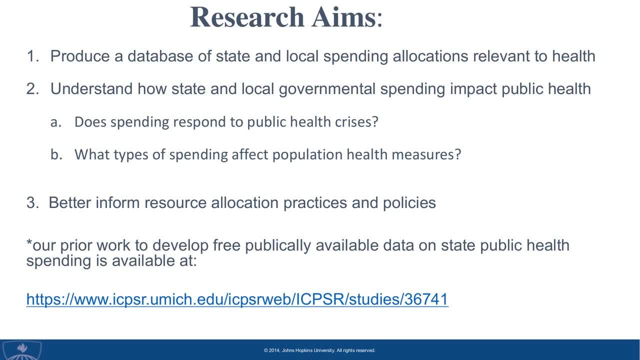 health And then, ultimately, long-term vision. that's number three. here, what we're aiming to do is use this knowledge and understanding and analyses to better inform how we're making our resource allocation decisions. I also wanted to just point out- at the bottom here there's a link to we're going to be talking. 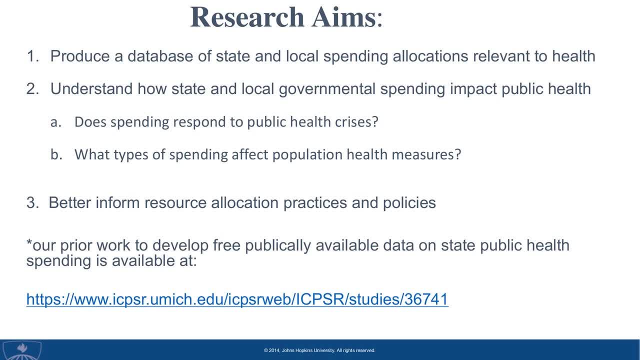 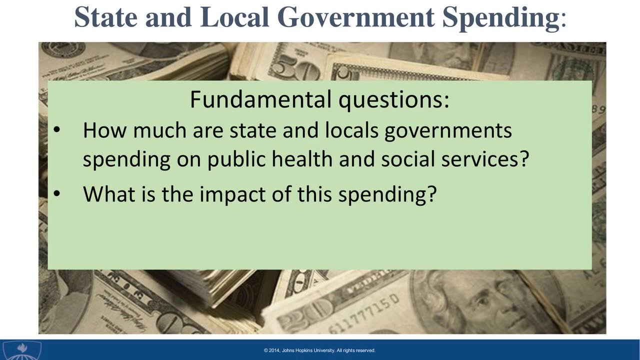 about some analyses we've already done on state public health spending And that is publicly available. There's a link here in case people want to view that data. So, fundamentally, what we're going to be looking at is one: how much are states and local governments? 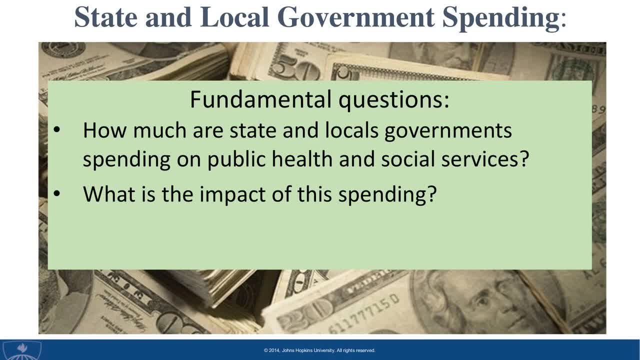 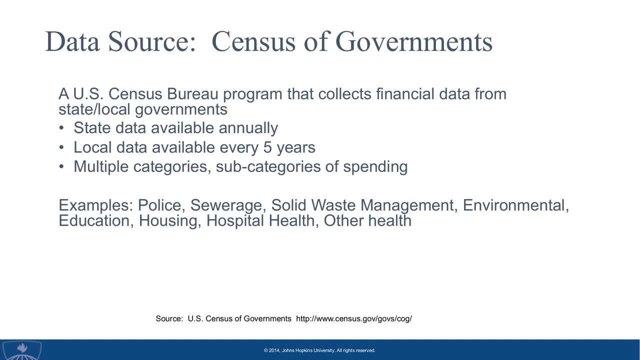 actually spending, And then two, what is the actual impact? So, first, to jump into our methods, so I want to explain a little bit, and maybe some of you are familiar with this. but what is our data source that we've been using? 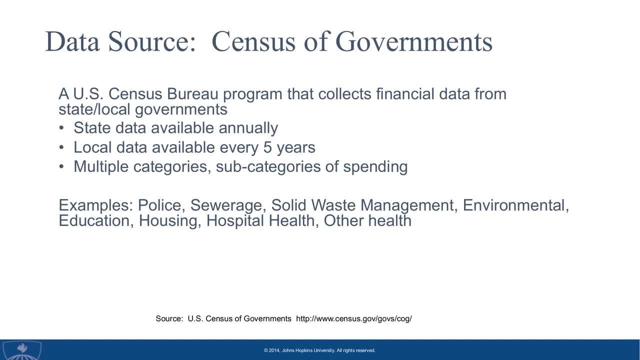 It's the census of government, And the important part is that it collects financial data from state and local governments. State data is every year And local data we have every five years, And then the other key piece here is that it's multiple categories, so you can see not. just public health, But these different categories, police sewage, so you really can get a better understanding of what states are doing. So I talked about this a little bit, but just again to give you a visual, to kind of make it clear because it can get confusing. is so the states report their spending data. Again, this is probably the state level Office of Management and Budget reports it to the census. Then the census actually uses the data that they code. they use it as code 32, is non-hospital public health spending. The census actually passes this information on to Centers for Medicaid and Medicare Services. CMS and they are actually the ones who do that national estimate of what the public health expenditures are for the whole nation. So you can see on the bottom, where we have the blue arrows, what our role was. We took that census code 32 data and we looked at it, line item, which I'll show you how. we did it and we recategorized and you'll see this. we're calling it the state health expenditure data set. It's a set of what actually states are spending on public health. I think you'll be interested to see what our findings were. So what we were looking at was, when we were doing our coding, we were using the foundational public health services, which I'll show you in the next slide, But what we were finding was that there was a lot of clinical services that were actually mixed in, so say, behavioral health care, or if a health department is running a clinic. These numbers oftentimes get all thrown in and coded in by the census, All right. So what we did was we disaggregated the census as public health, that code 32.. And so really we think the numbers are going to skew what we're looking at, because we're thinking that we're actually spending more on public health- population-level public health activities- than we actually are. So what we did was we disaggregated the census estimates and went state by state to look line by line. We used this. hopefully this is familiar to many of you. this is the foundational public. health services coding framework. And again, Washington State. Washington State is using this. They're doing a chart of accounts project to again look at what we're spending on public health and trying to understand better the impact of our spending. So I think Marie will be talking about that. But this is our coding framework that we were using. So every line item we are then coding which bucket this is going to go into And you can see on the left side. here you have under the green background what is considered under the foundational public health services as being public health. We also coded on the other side- on the yellow, on the right side, what is non-public health in terms of other health services. So, for example, environmental protection, behavioral health or the big chunk of it, was a lot of clinical services. So then we did a descriptive analysis about what we found, And I think this key point to this graph that's really important is this pie chart: the green here, When we recoded, this is from 2000 to 2013,. state-level spending. 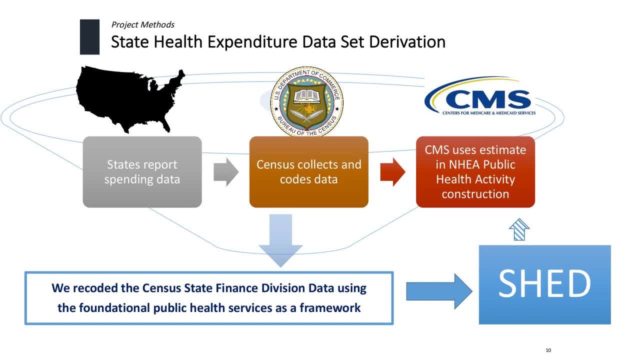 We found that what the census is actually counting as public health, only 39% of that, according to the foundational public health services, would fall into what we want to consider population-level public health spending. So why is this important? It's because the national estimate is actually, even when we think it's so small, the number 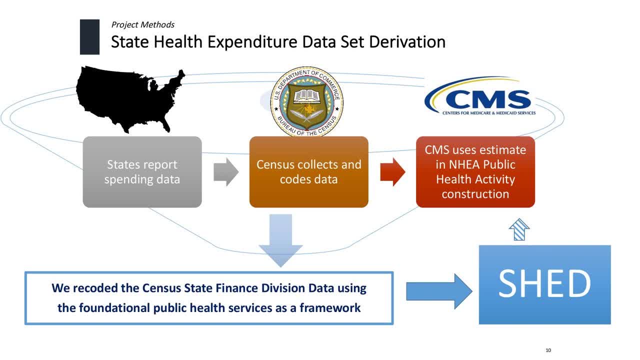 we're spending on public health. it's actually the real number is even less than half of what the national number is. when we think about how we're estimating what we're spending on public health, And then, clearly the important piece- what is the impact of that spending? 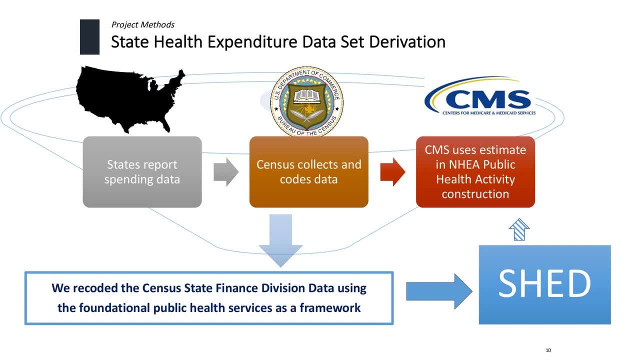 So you can see on this pie chart, the next biggest chunk from public health is actually behavioral health. But again, this is important in the sense that the denominator we're using in our public health spending is wrong and that it is including lots of other valuable services, but they're. 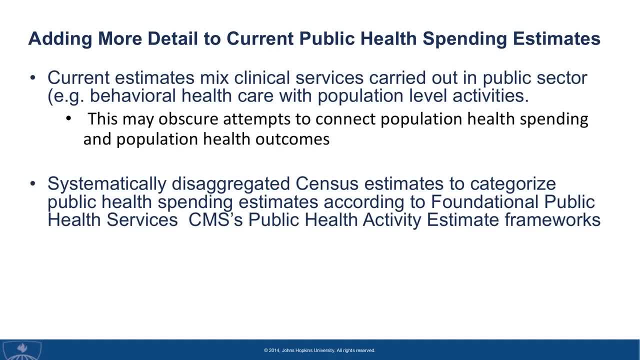 just not population-level public health. So we find this is a really important point that we're trying to share and disseminate with people to understand when again, to allow us to better understand the impact of actual population-level public health spending- Another thing that we've been able to do with this data that Dr Deschai will get into more. 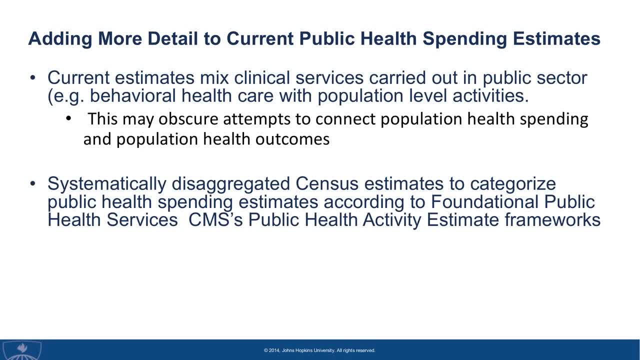 but we're also in addition to looking at total public health spending. we can also look in different categories. So you can see in this slide there's maternal, child health, chronic disease and this is state-level spending Again across these different years and you can see that it stayed fairly stable in. 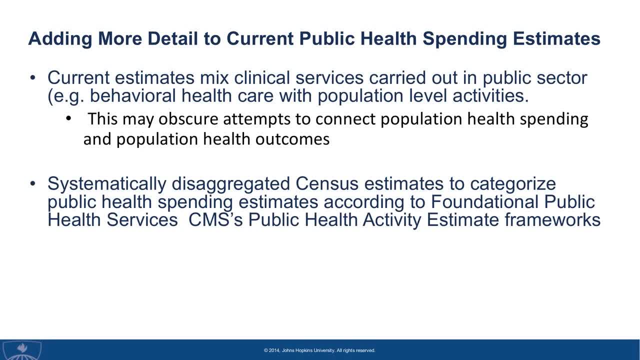 each category And again, Dr Deschai is going to be getting into more depth about some specific spending levels. but you can see that the ability of this data for us to look at trends over time and share this to get a better understanding of what we're spending. 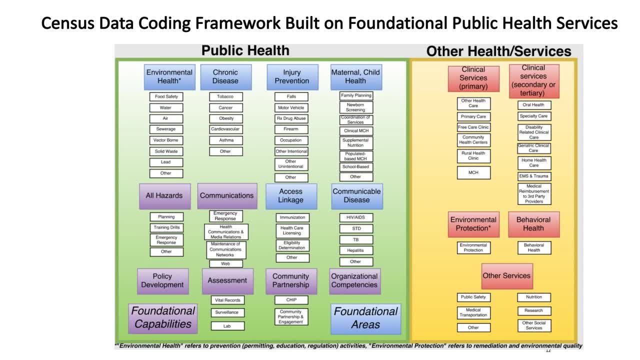 So next we're going to go into analytical results and I'm going to pass the torch over to David Deschai to explain this. Hi, This is David Beth. can you hear me okay? Yep, I can hear you, Thanks. 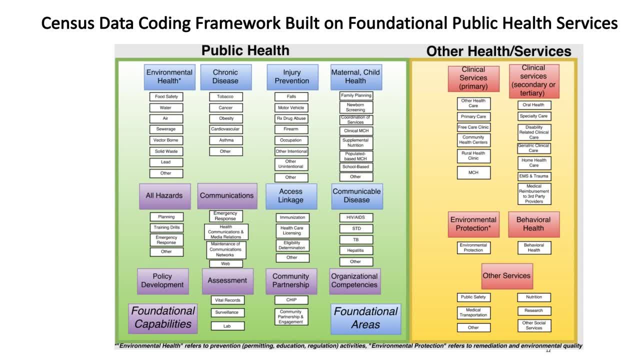 Okay, Can you just go back one slide about the trend data, And I wanted the audience to look at the flatness of the trends and really be a little curious, because after all, the trend starts in 2008 during a major downturn in the national economy. 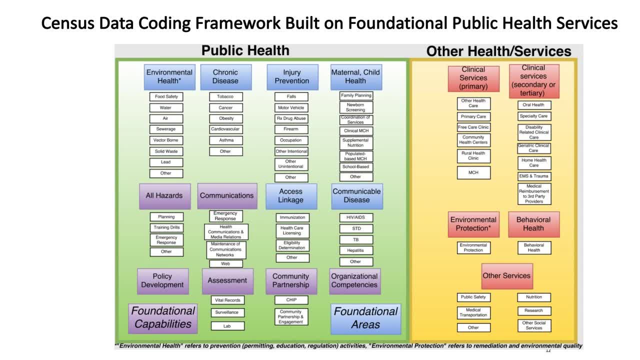 and the state economies, And yet we don't see these various buckets remaining Okay And we don't see these various buckets respond to that spending crisis in state budgets. And the other issue that I want to point out for where we're going with this is noticing 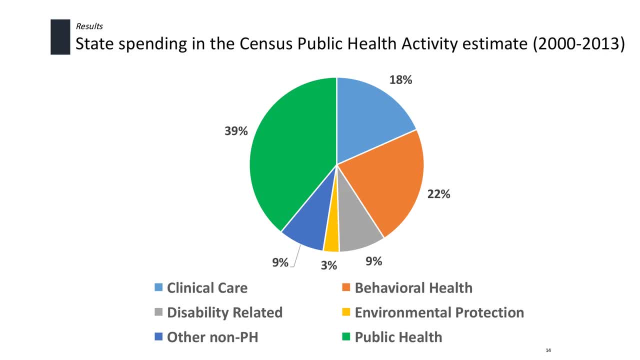 that it doesn't rise at all. There are obviously within each state there are rises and falls, but the national-level trend doesn't seem to respond inside these buckets, Even though the country is facing some crises in drug deaths from opioids as well as other. 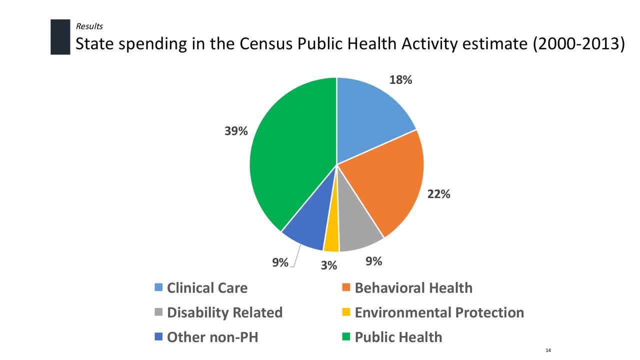 mental health issues, And none of these particular areas other than chronic diseases maybe, would be responsive to that. But I wanted the flatness of these trends to be curiosity-provoking. And now let's just go on to the two questions that our analysis is trying to answer. 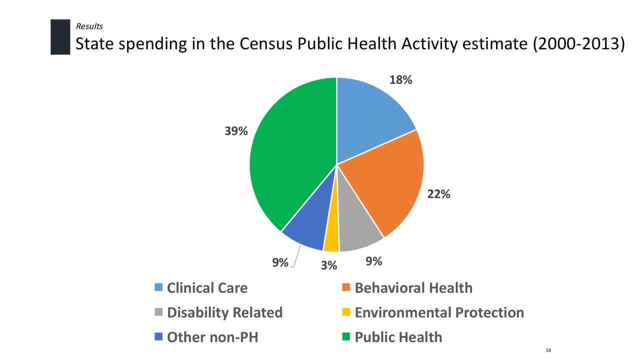 Does the spending respond to health problems? And then the second question: does the spending improve population health? Next slide: Okay, So these are data from the CDC and we plotted. these are cost-specific, age-adjusted mortality rates in various states. 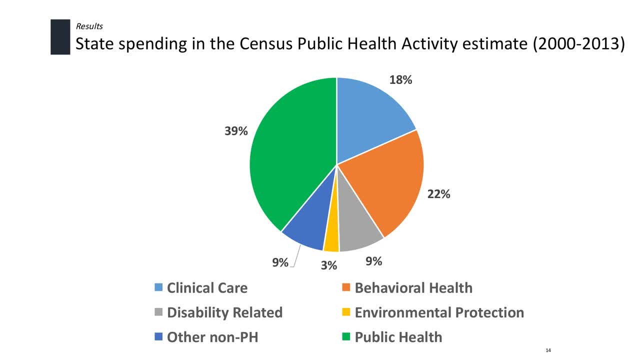 You see alcohol in South Dakota. You see a trend from 2000 to 2016.. I think persuading most of you that during this period, South Dakota appears to have an emerging problem with alcohol. that's coming up around 2012 to 14.. 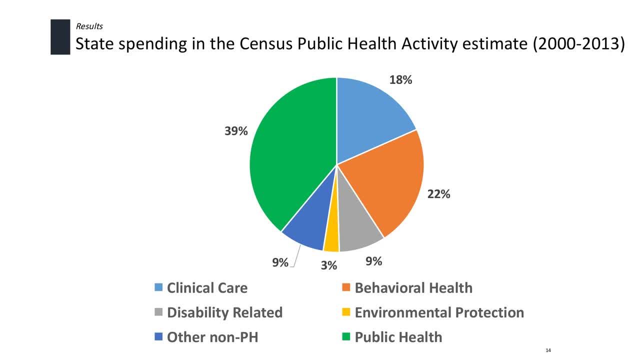 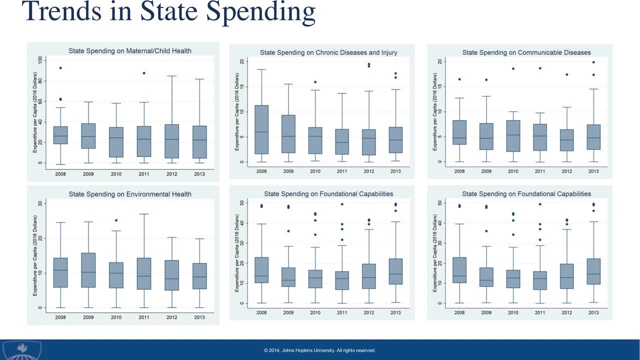 Idaho. You see, You see an emerging trend somewhere around 2010 and 12 in suicide deaths. Alabama, like many states, is seeing the emergence of a drug-death epidemic of 13, 14 years ago. You can see it start to trend up. 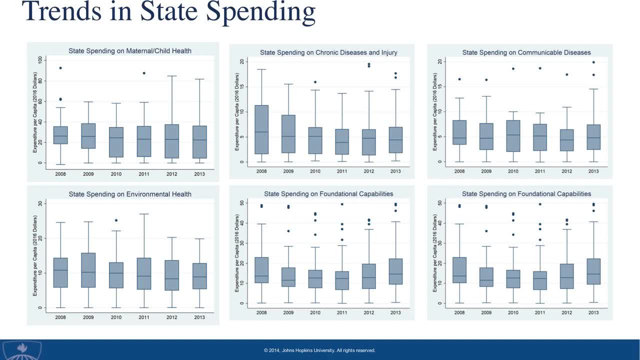 And different states have these different uptrends at different times. So the analytical question is: wouldn't we want to live in a country where state health departments saw trends like this and reoriented some of their budgets to, let's say, drug-related deaths? 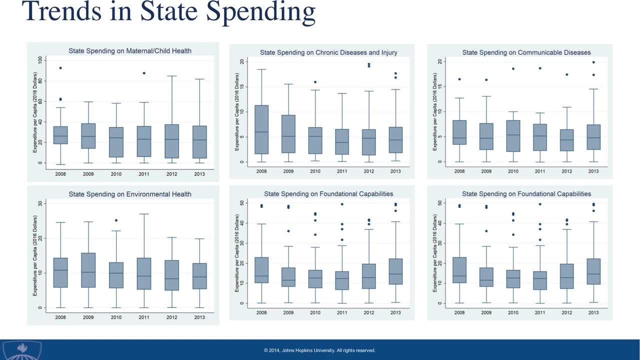 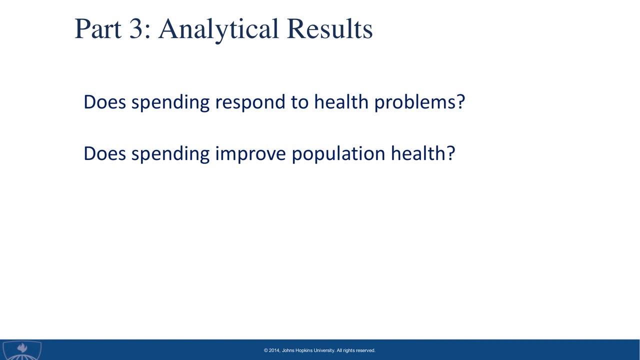 So we're going to have to do the preventive work on these problems. Obviously, these problems will naturally lead to psychiatric utilization. These reflect individual needs and certainly, whether the State Department of Health does anything, you'll see extra claims going to private carriers, as well as Medicaid and Medicare. 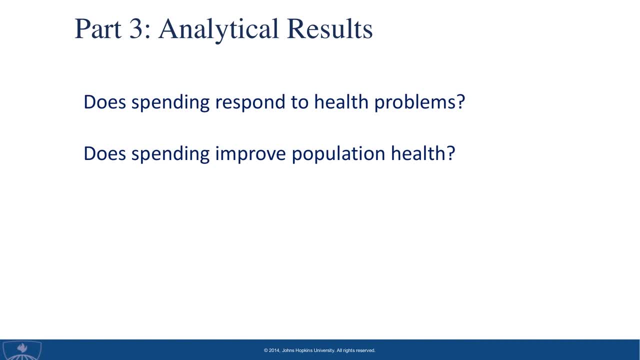 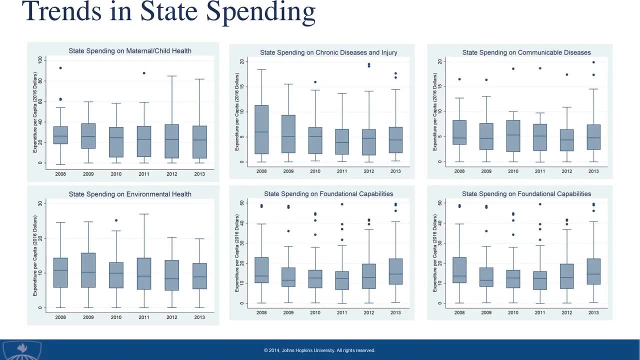 But the question now is public health. Does public health have any tools in its toolbox that can respond to these problems? Can they respond to these crises? Can they start to bring in tools to do prevention of alcohol, regulating alcohol outlets, doing early detection of people with mental health problems, et cetera? 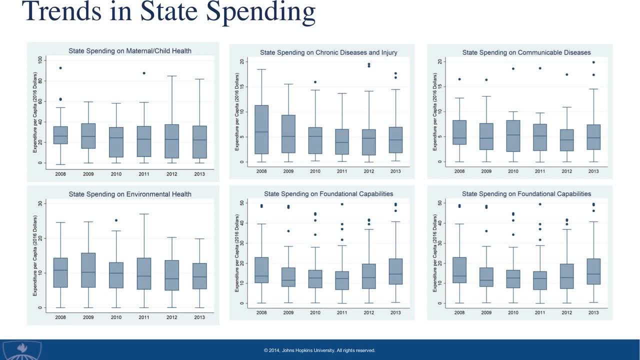 So I'm of the mind that, yes, there are tools in the toolkit And the question is: do the states have the ability politically to shift their funding? And that's the question we're about to look into, And we're at the early stages in this question. 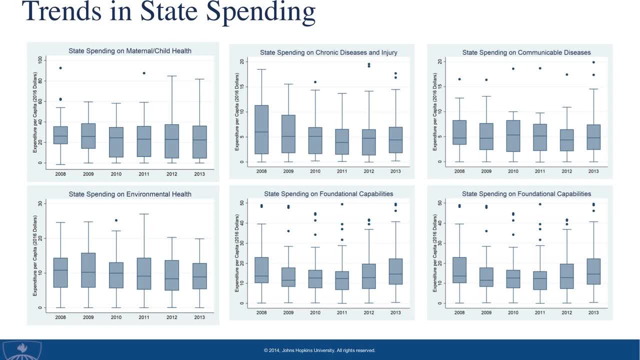 So I'm going to turn it over to you Before we move on. if you look at these trends, you're not going to expect South Dakota to shift its spending every single year. If you look at South Dakota, it's not going to look at 2008 and say, oh, we had this tiny. 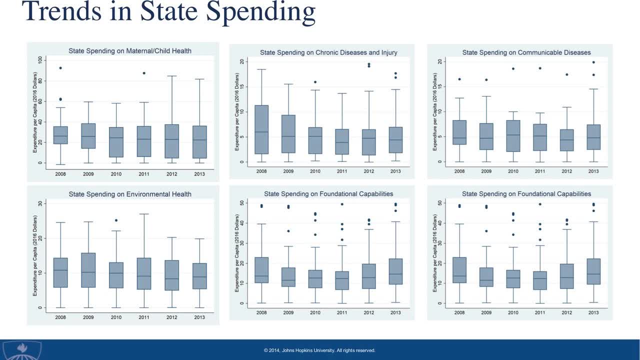 little uptick, Let's shift our spending. And then in 2009,. oh, we hit a little downtick, We're going to shift our spending. So that's really not it. But sometime between the early 2000s and the 2010s, South Dakota is going to shift its 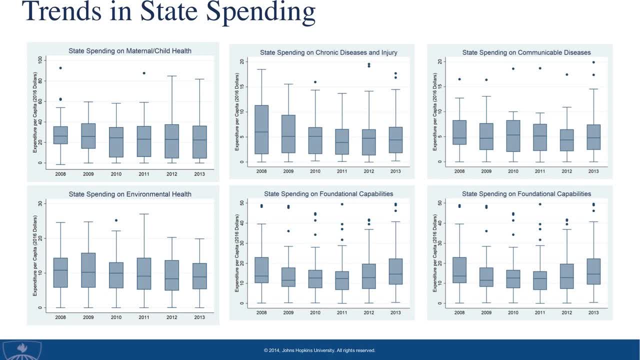 spending. So we're going to shift our spending. We're going to shift our spending And then in 2018, South Dakota, we would expect to respond. So that's the type of data that we would like to the question we would like to ask. 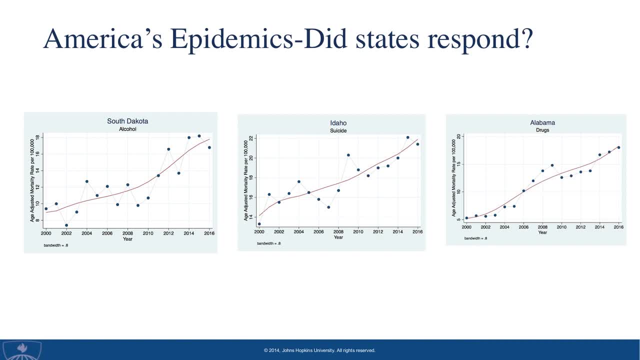 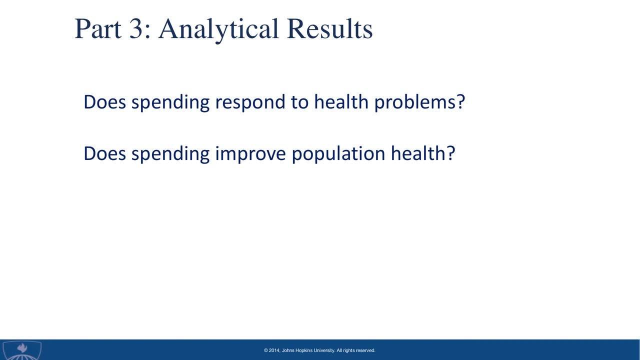 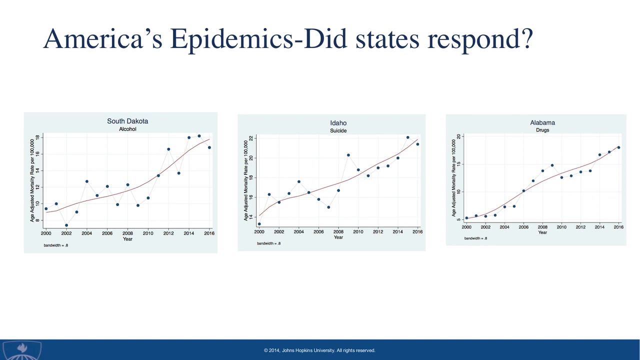 And we're- let's show you where we are right now in the next slide in our analysis. So this is a scatter plot of the change on the horizontal axis. It's this change in AADR, that's age adjusted death rate. That's the annual change. 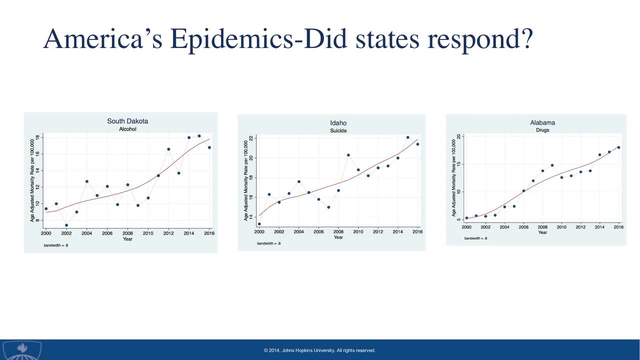 And if you look at where zero is- zero is kind of towards the right- You can see that on a yearly basis there's a lot more downturns in all of these causes than there are upturns. There's much more going on on the left by various causes. 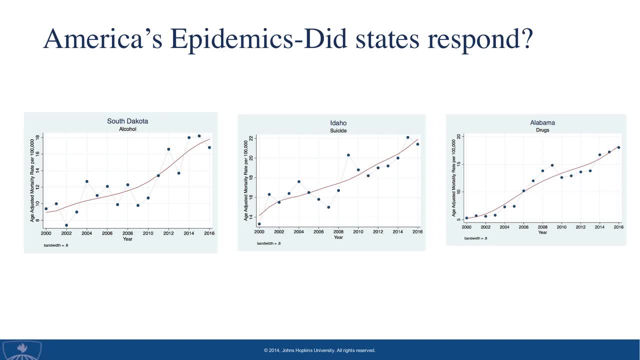 Really exciting news If you are excited about cardiac disease going down, you see lots of downturns in cardiovascular disease, strokes, diabetes. There's a lot of good news in America about states experiencing downturns in age-specific causes of death for cancer, heart disease and stroke. 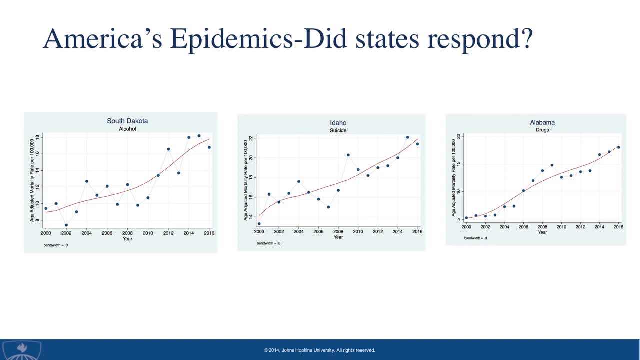 So we're going to shift our spending. We're going to shift our spending. The next slide, please. So here's some of the data that I have has shown that, and we've started to have a lot of evidence in America regarding the initial effects of stroke. 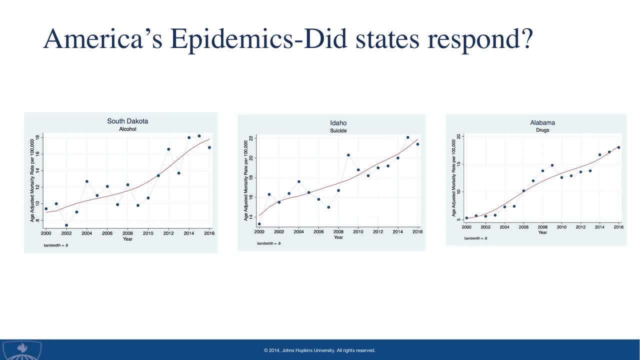 So on the right-hand side we see the positive results of the change in the age adjusted death rate going down And this is the number that shows the seriously low response rate of patients to stroke on an annual basis. On the right side, the colors that you're seeing are a little bit more attuned to drugs. 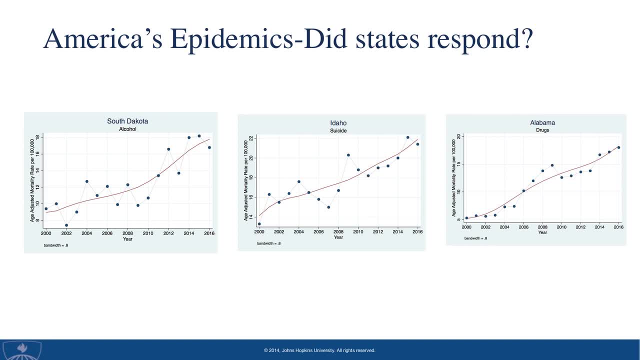 in the yellow, suicide in the blue and alcohol, The more uptick on those three causes and this is something I think we all know. On the vertical axis, you're seeing the change in state fending, And again on an annual basis. some states are moving their spending down and some are. 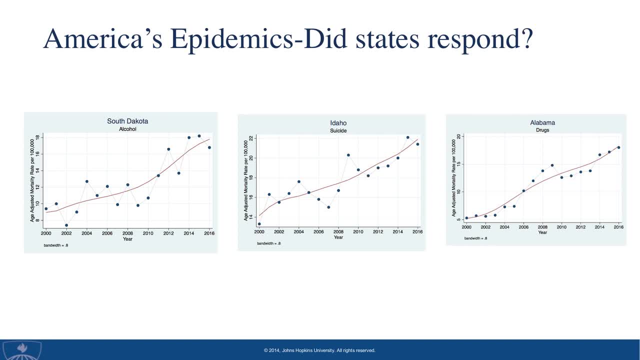 moving it up. But overall across this scatter plot there's no systematic change that's been made to kind 45-degree line, Our hypothesis that on an annual basis people will see their death rate go up last year and one year later move up their spending. that is absolutely unsupported here And, as I 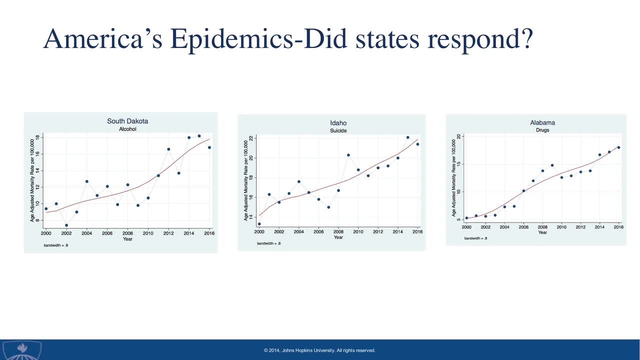 said earlier, I wouldn't expect states to be, you know, moving their budgets around year by year because, as you rightly infer, an annual change in a death rate is a lot of noise and not a lot of signal. It's not really clear that one has to change your spending on an annual basis, And 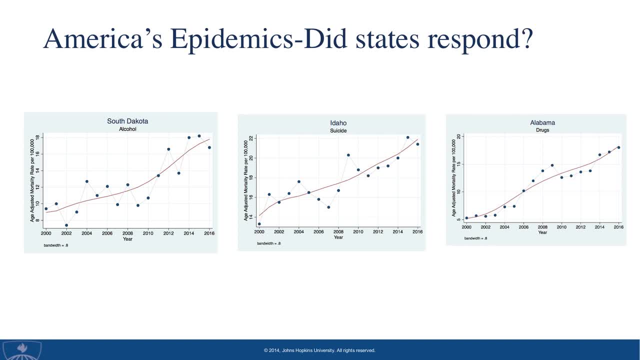 you know, this result shows that they don't. The next slide shows just the focus on alcohol, drug and suicide, And if your eyes are careful, you can believe what I know, which is that there's way more upturns to the right of zero than there are downturns to the. 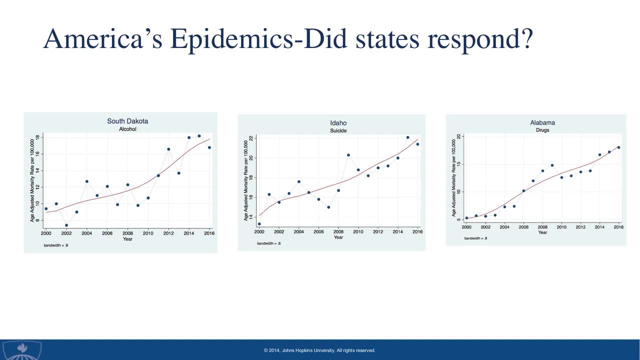 left of zero, So you can see more dots on the right of the slide there And the left, showing what we know is that there are more, that these three causes of death are going up in the state for the last 15 years. But again, are states calibrating their spending on? 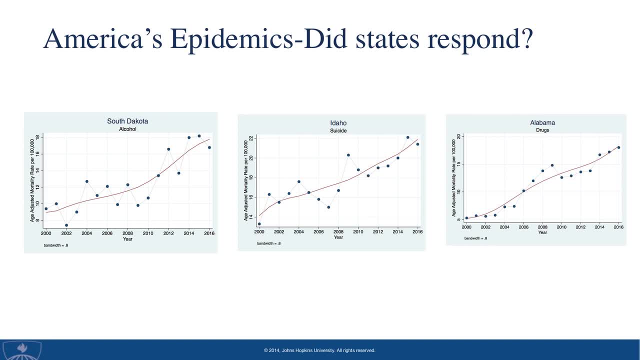 an annual basis. Is there any type of a regression line that's sloping on the 45 degrees, where a change in death is accompanied, one year later, with a change in spending? And the answer is no, there's no correlation. So, finally, besides these, 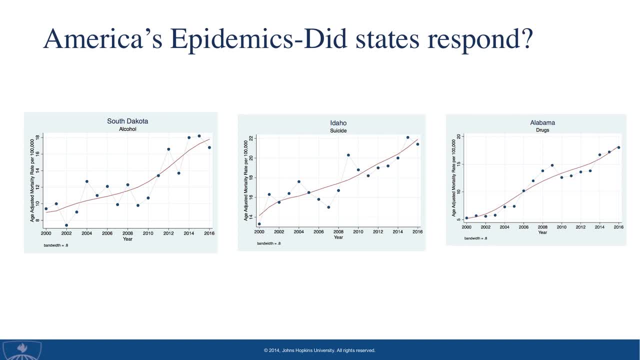 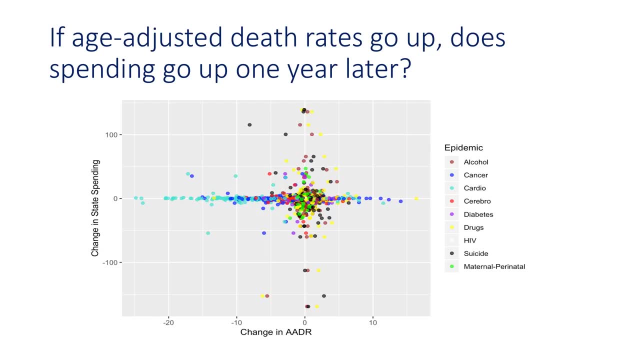 graphical versions. the next slide shows the statistical regression model where the dependent variable is just the behavioral health spending, because we wouldn't start to move the entire state health budget related to alcohol, suicide and drugs. We would just expect us to change the behavioral health spending, And so we look at the first row whether there's a correlation. 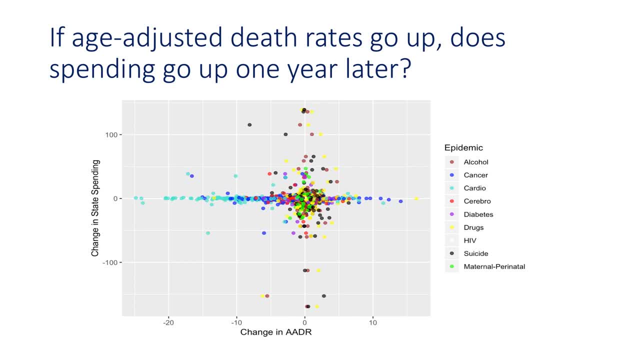 between the age-adjusted death rate from alcohol, suicide and drugs and there's no statistically significant correlation, except in one model on the far right, where it goes the wrong direction, where, if a state is having problems with alcohol, suicide and drugs, 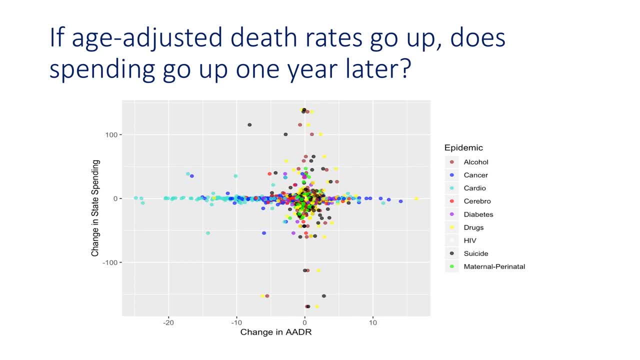 it's actually less likely to spend money on behavioral health in the subsequent year. And again, this isn't really the right way because this is testing it on an annual, year-by-year effect. State median income does predict spending The third row down. 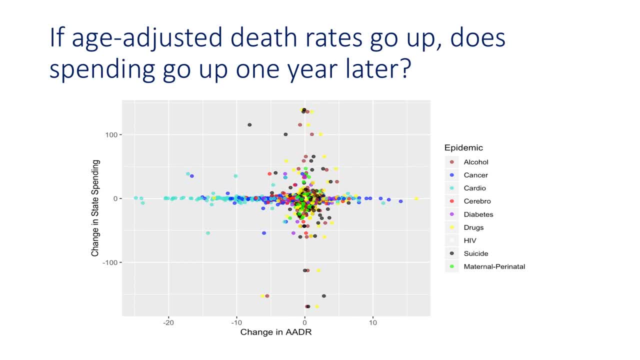 richer states are able to increase their spending on behavioral health, And in some models we um urbanicity is predictive and in other models, being urban reduces the spending. So we're still working on this and we're happy to take your feedback on it. So this is early on. 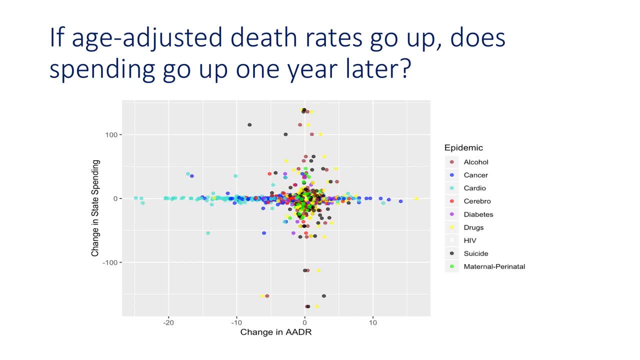 the question of do states calibrate their spending? And, as you can tell, I'm not happy with doing it on an annual basis. What we're working on doing is flagging start of an upturn on these conditions. When exactly did South Dakota's suicide? 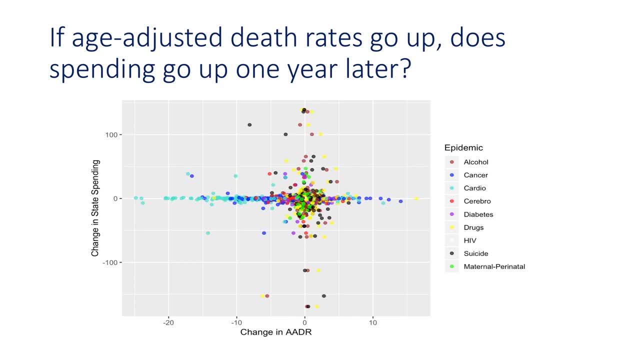 epidemic start? When exactly? would you know? North Carolina, We can time the time at which the state epidemiologists would have said: you know, governor, I think we're having a problem now That occurred at different times in different states and we wanted to tie in to say, you know, were they able to locate the 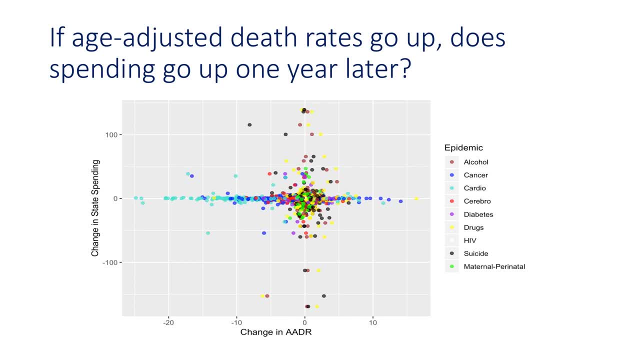 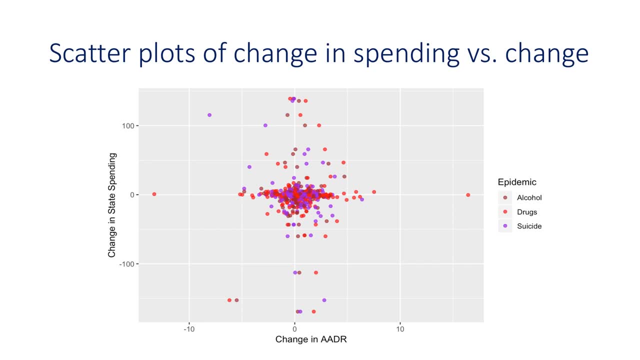 start of their problem and then subsequently alter their budget. Now I hope the hypothesis bears out. I want to live in a country where the governor finds public health crises and is able to shift spending towards them, but I have my doubts as of today. We'll see what's coming. Okay, let's move on. 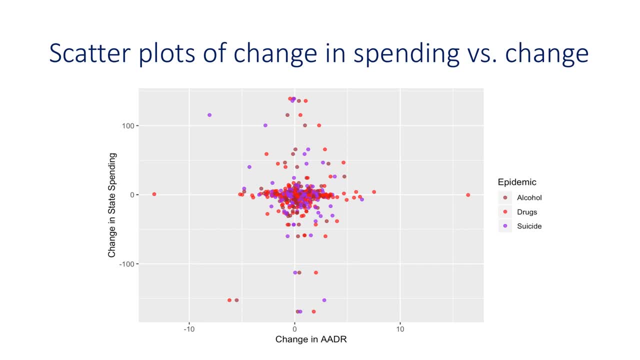 to a new question Next slide. As Beth said, we are blessed with data on multiple sector spending and we want to ask the question: how do multiple sectors of spending in the control of governments, local governments- affect health? So let's show you how we're. 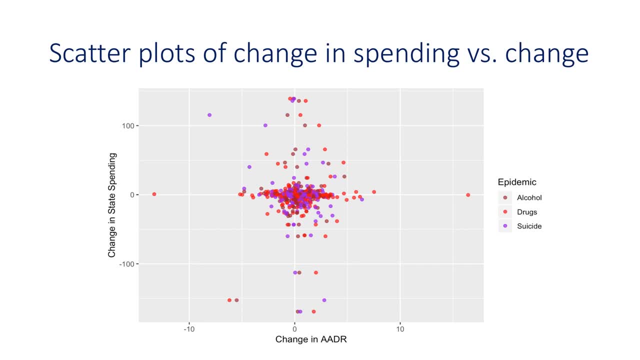 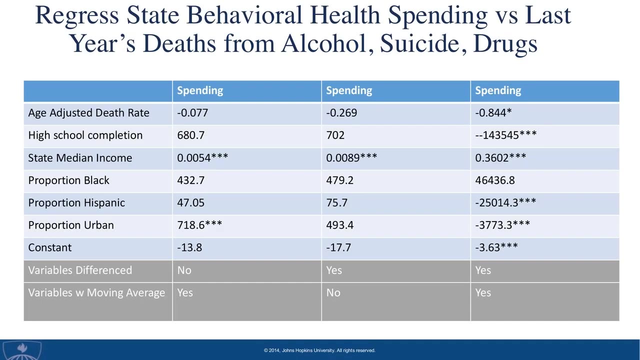 approaching that Next slide. So, because of this wealth of data, we have various buckets of spending In the bulleted list here shows you the spending. It also shows you our current classification of three large organizing categories of this spending. So understand that this is an organization that has a lot of 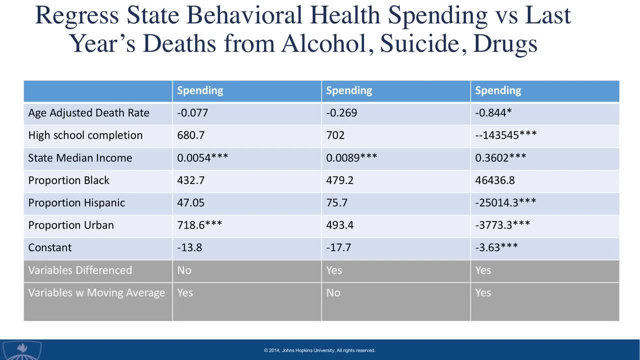 social spending. We put non-hospital health, which is our main focus. This is what we're calling a lot of public health mixed in with some clinical services for behavioral health, as well as STD clinics and other non-hospital public sector spending. This is not claims. 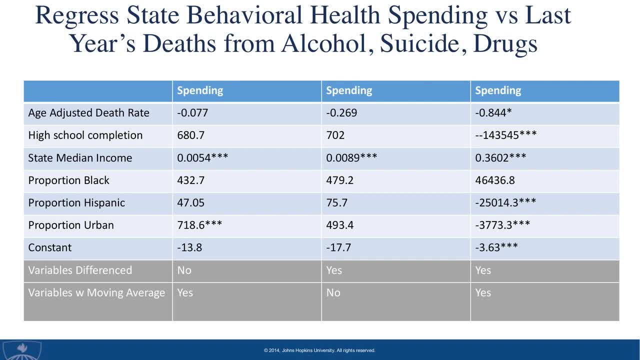 This is not Medicaid. It's what comes into the state budget. That's the first bullet up at social spending. But we're mixing in with that spending by states on public welfare, education, life care and health care. So that's the first bullet up at social spending. 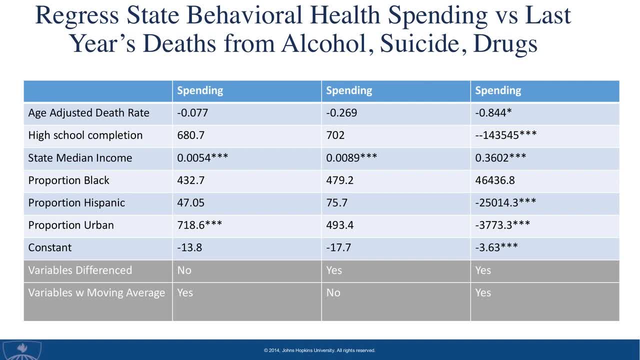 So here you can see the numbers that we're seeing. I'll show you the last one. This is going to show you the total money spent on medical, social, medical health and social systems. In addition, we're focusing on community planning, public health, social public. 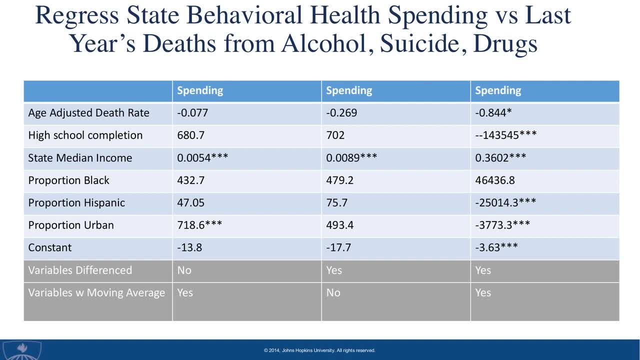 health and the state of Colorado. So in many cases it's all based on the state's money spent. It's no longer put into the public health budget. We now have the state's financial, We now have it all in the state budget, our national budget, our. 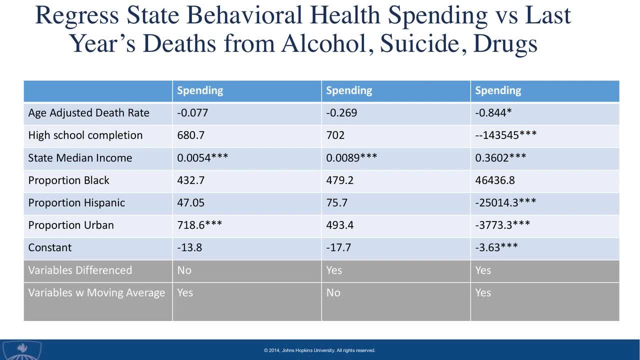 state's federal budget. So we're not just using the state budget in order to get all that money spent. we're using the state budget in order to get our local state budget and our local state budget. So our state budget is really based on the. 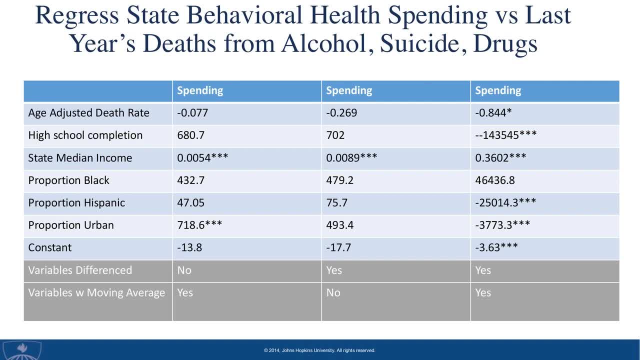 past fiscal year numbers, And so at this point in time, we've actually spent a ton of. we spent a long time trying to get the data to tell us what variables went together, using a method called principal components or factor analysis, and it really wasn't coming together statistically, and so we started. 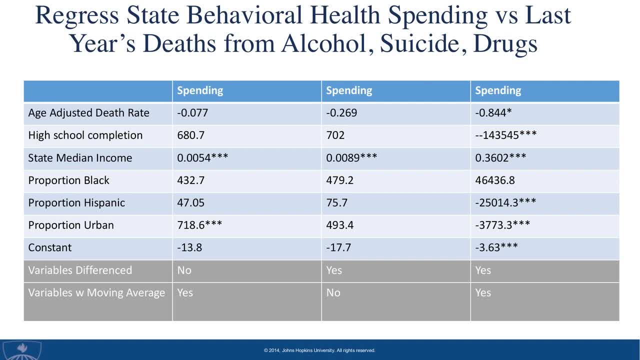 interviewing state budget planners to see how they thought of the problem. and- and this classification is where we are- are now at the bottom. we have a fourth indicator variable, which is a mix of poverty, unemployment and total county revenue. that also definitely affects the spending, but it also we know that the 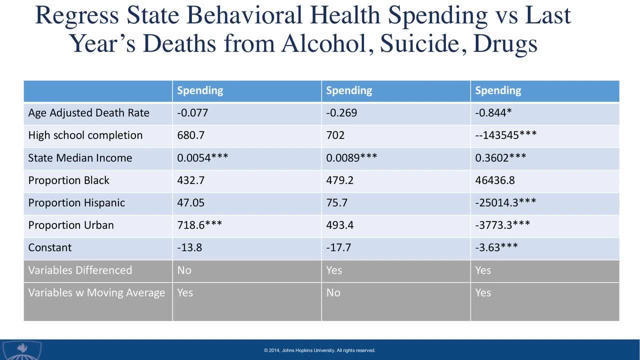 economy can affect health directly. so we're going to take these four latent areas, the three spending buckets and the economic stress category and try to ask the question: are these categories of spending and economic stress related to health? next slide. so the method we're using is called structural equation modeling and it is a 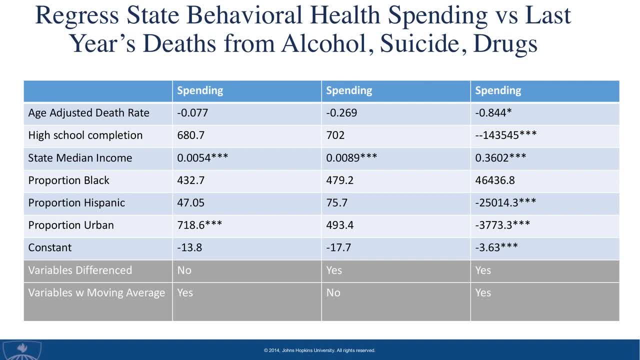 way to assess relationships between things. we observe multiple indicators and then these categorical, latent or unobserved variables that I've shown you in the prior slide. the exogenous measured things we have are spending. we have measurements of life expectancy at birth. we have measurements of poverty. 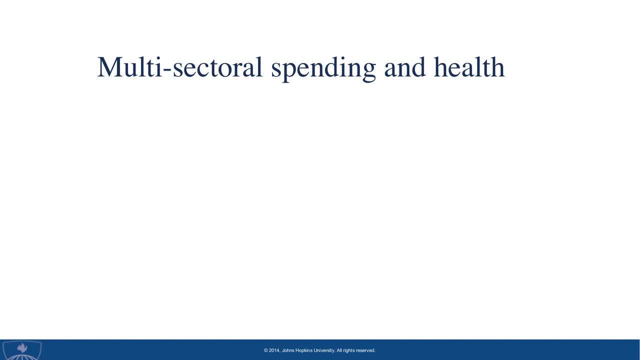 unemployment and government revenue, and we're going to draw a picture in the next slide which puts things like that in rectangular boxes because we can actually have indicators of them in the data. we're going to use circles or ovals to talk about these latent structures and these will be the county spending. 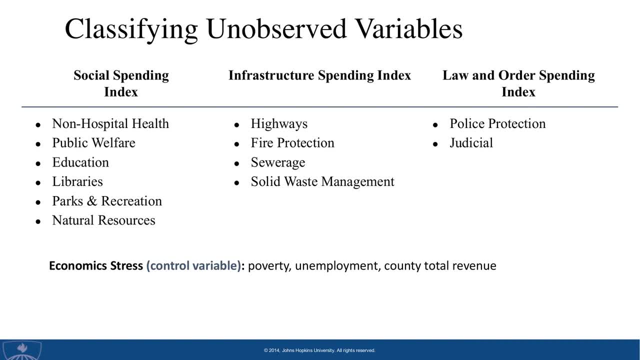 index and the economic stress index. so that's what you're going to see in the next slide is is boxes of real measured things and ovals of latent things. so, if you can for a moment is- it's complicated, but if you keep your eyes in the center, 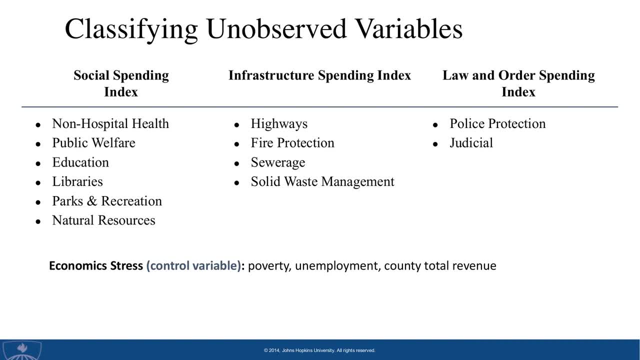 it's simple because there's only five things in the middle. there's these four ovals of these latent categories: infrastructure, social law and order, and economic stress, and then there's this rectangle of life expectancy at birth. so, fundamentally, the the questions can ask you know what is the effect of these? 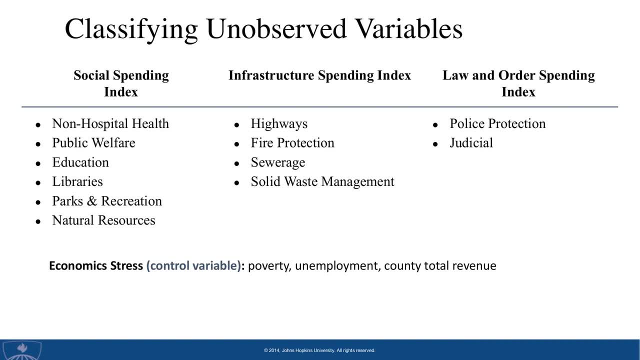 four ovals on life expectancy at birth. now I'll give you permission to go and look at the complicated parts on the outside where we say we are going to measure infrastructure as a summation of levels of spending on sewerage, fire protection and solid waste management. 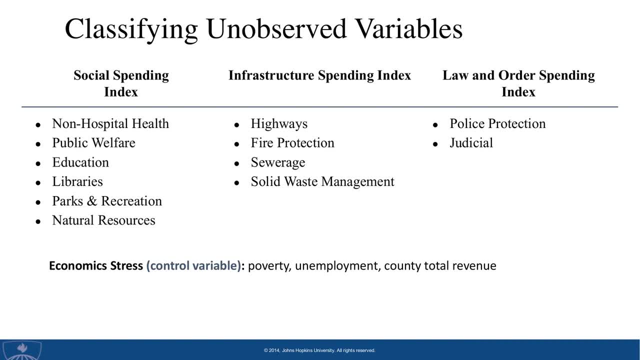 highways. we're going to measure social spending as a mix of the six things you see in rectangles and law and order on the three things you see in the yellow rectangles and so on- now almost invisible, uh, and the ones that are coming soon are those little numbers, which is what the 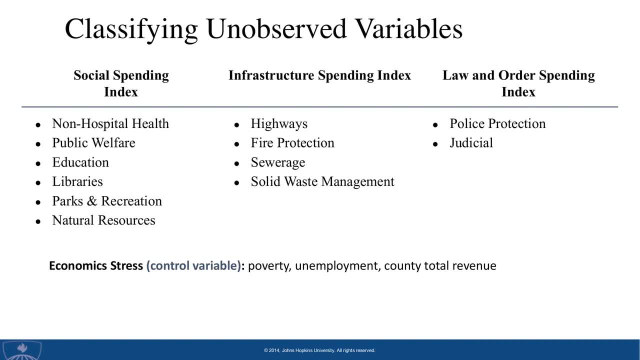 model fits out, and I'm going to get to that in about five to six minutes, but I wanted to let this soak in for a second and in the next slide we're going to focus in on the top left to show you know our model of that oval called 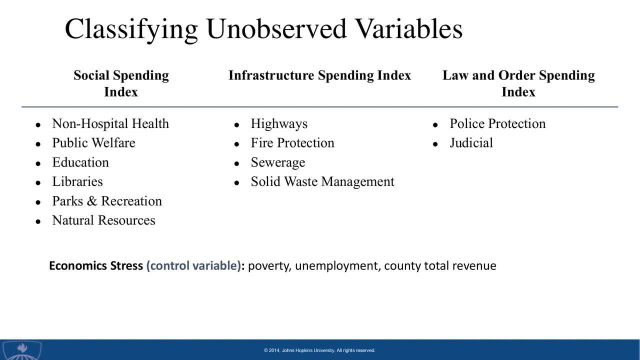 infrastructure. so next slide. what you're seeing here is the blow-up of the numbers of infrastructure. and is that the contribution of these four measurable things of sewerage, fire protection, solid waste in the highways? each of them has different weights in a, in a measure of infrastructure. the weights say that this is mostly what the 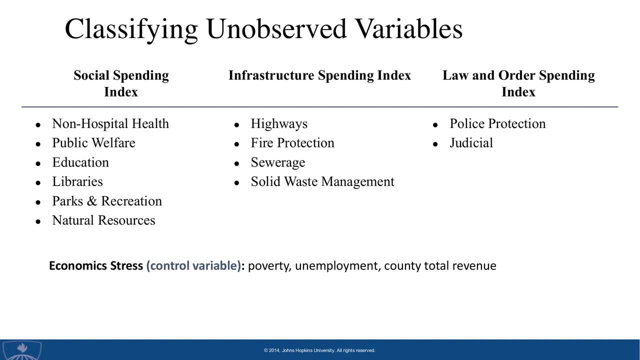 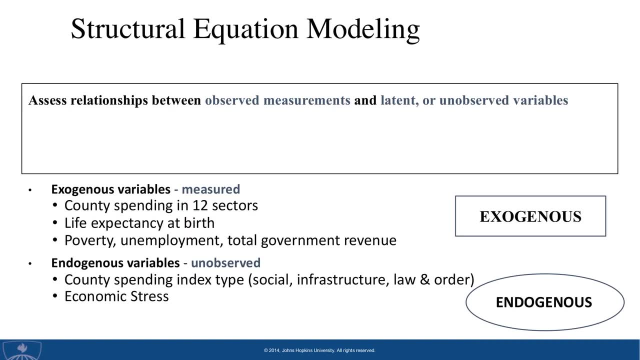 data wants to do. it doesn't say anything other than this is how one would go about getting a measure of infrastructure that combines sewerage, fire protection, solid waste in the highway. but these four indicators come together in this latent category of infrastructure in that specific way in. 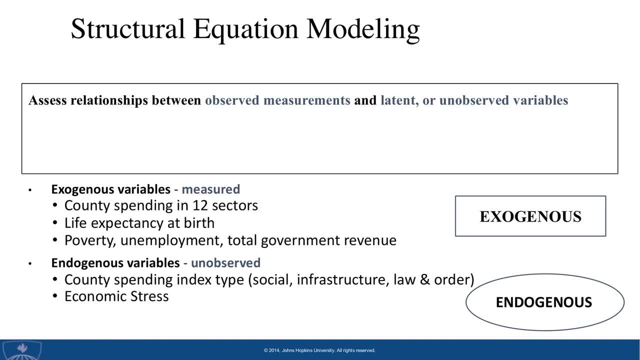 the estimate next slide, and this is a measurement model of an indicator of social spending and it's saying that, you know, relative to the natural resources spending, health counts two point four times as much as the natural resources spending and the education counts, point two, five as much. with these different weights, these 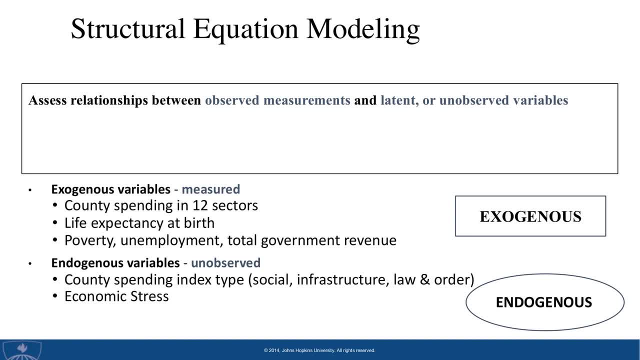 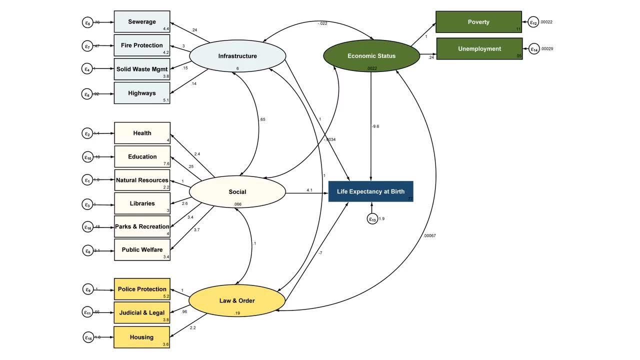 weights are not just how much do these things go together, but the model says these things have to both go together to predict social spending in a way that predicts life expectancy. these are, these are the health relevant amounts of spending weights. so that's what the measurement model is trying to say. next, 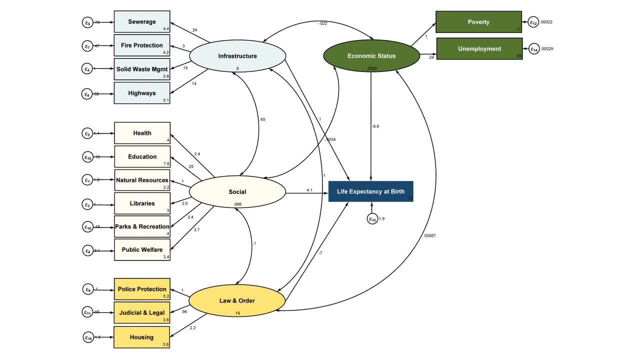 slide. the last idea. this is how we we found the the three measurable factors: the police, judicial and legal spending and housing spending. this is how they weigh into an index of law and order. next slide. so these are the three measurements of social spending. we have got a basically. 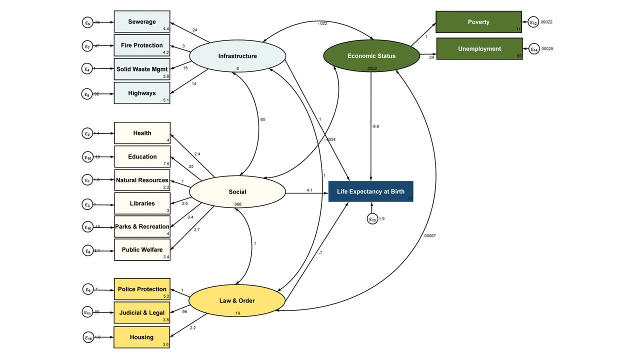 a propensity to want to spend on infrastructure, propensity for social spending and propensity for law and order. So each of our counties rates differently on these blue, tan and yellow ovals. Some counties do a lot more of one than another and it's the propensity to spend having large 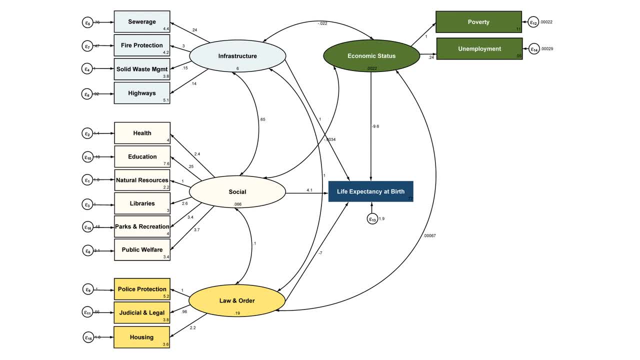 values in these indices and indicators of social spending that we can now ask: does having a high propensity for infrastructure affect your life expectancy? same as social spending and law and order? And that's where this final slide will try to tell you the answers. 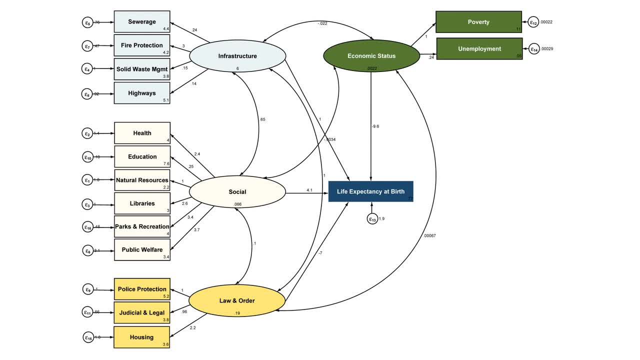 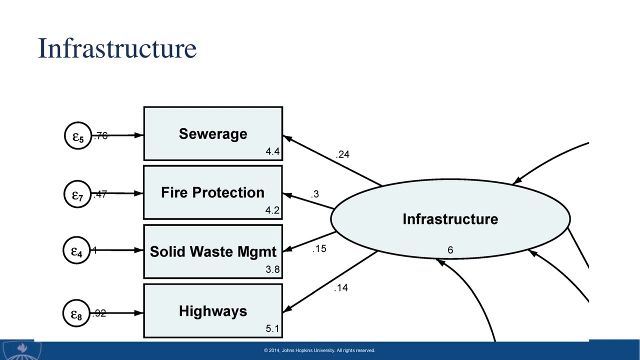 Next slide. So back to where we were, and again I apologize for the size of the numbers, but if you can see an arrow between infrastructure in the blue and life expectancy in the blue rectangle, there's a diagonal arrow with a one next to it. 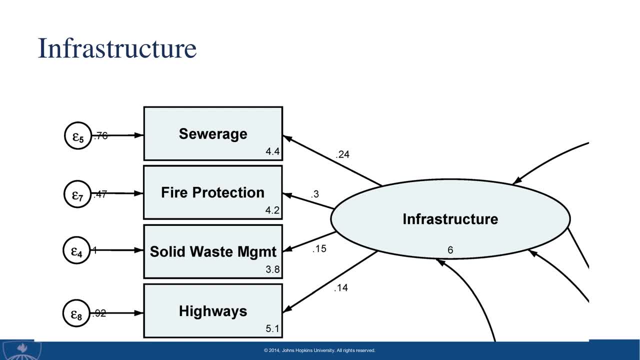 So that's the reference relationship And it says that you know, we're just going to count this as the reference and compare everything else to the relationship between infrastructure and life expectancy at birth. And now I'm going to point at the arrow between social and life expectancy at birth, and you 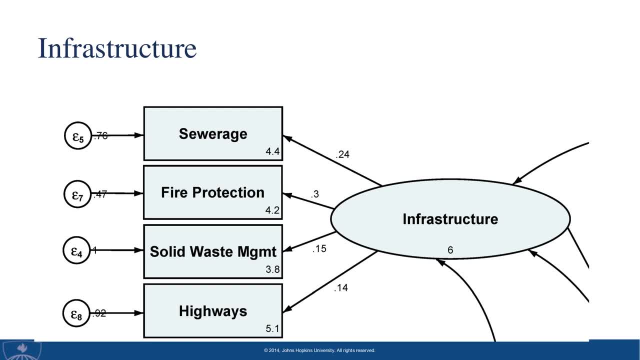 can see a 4.1 relationship between social and life expectancy at birth. That's a horizontal arrow that you can see and that says that, relative to infrastructure social spending propensity, That propensity has 4.1 times as much effect on life expectancy at birth and it's going. 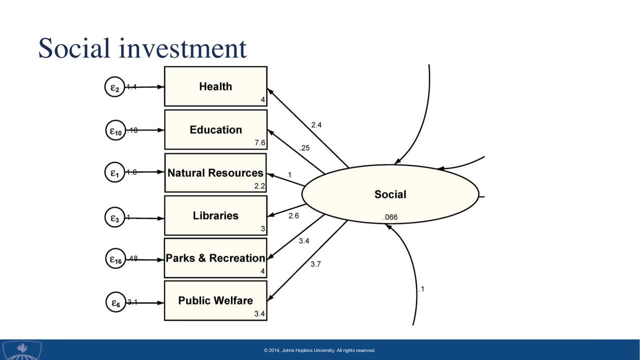 in the positive direction. It increases much more than infrastructure. The law and order spending value is negative .7,. you can see that as a diagonal, pointing diagonally up from law and order to life expectancy at birth, And that says that, relative to infrastructure, law and order spending goes in the opposite. 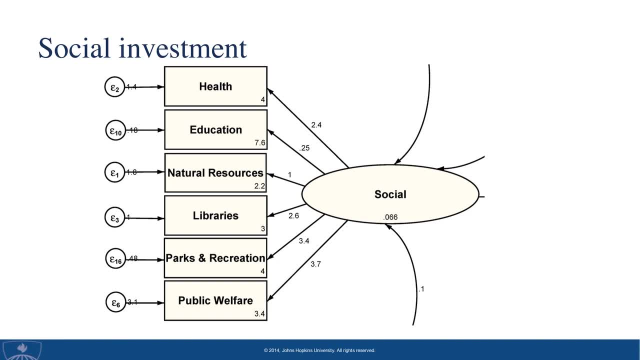 direction. So that's the reference relationship between social and life expectancy at birth and we can see that as the reference relationship between social and life expectancy at birth And we've done these models so that life expectancy is measured three years after the spending. 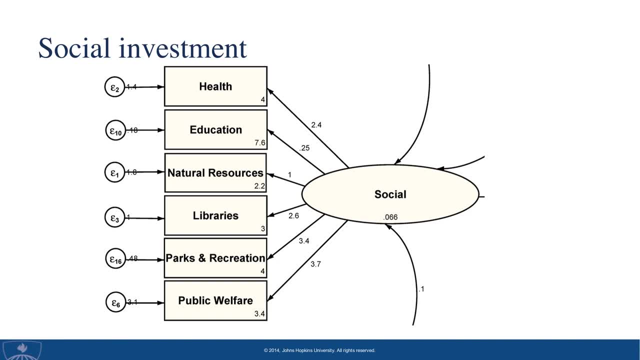 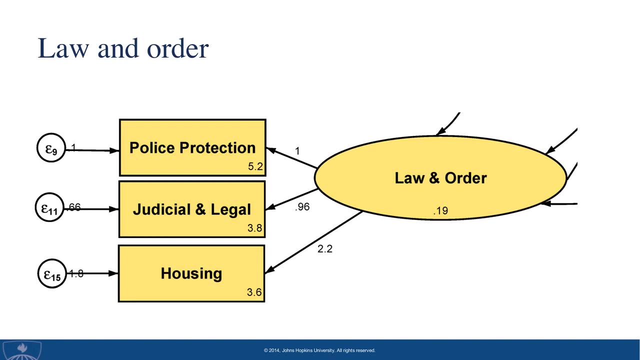 because obviously the spending doesn't work immediately, And we've changed it up. We can measure the life expectancy at various delay intervals and we pretty much get the same result. These three main results are statistically significant and the goodness of fit in the 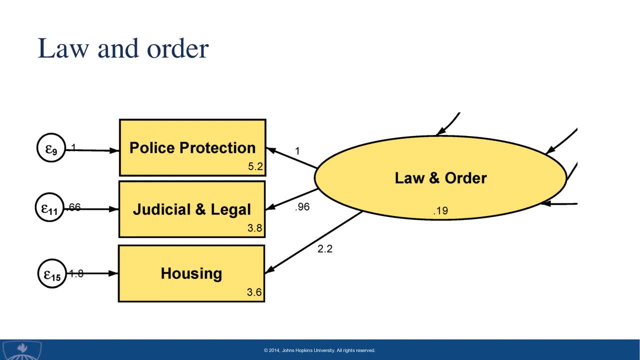 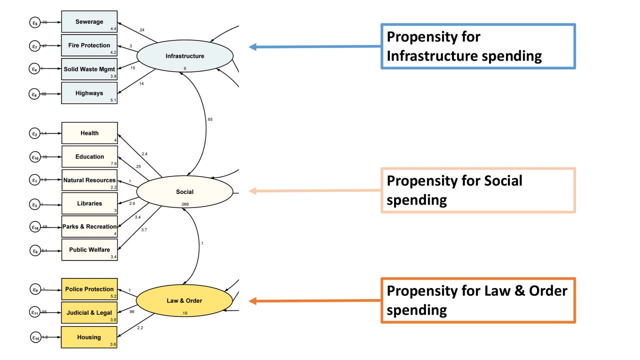 model is overall meeting the standards Okay. The last thing to say is that economic stress is bad for life expectancy at birth, just repeating what we all already know, that poverty and unemployment, and you can see that as a negative 9.6 relationship between economic status and life expectancy at birth. 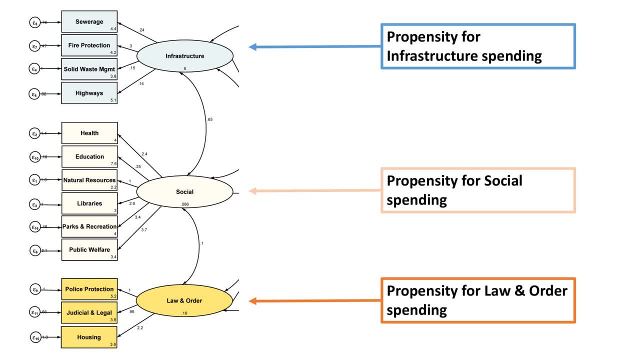 moving straight vertically down from the green oval to the blue life expectancy at birth. So this is a structural equation model that tries to test whether life expectancy at birth is bad for life expectancy at birth. Here buckets of spending outside of health are related to life expectancy at birth giving. 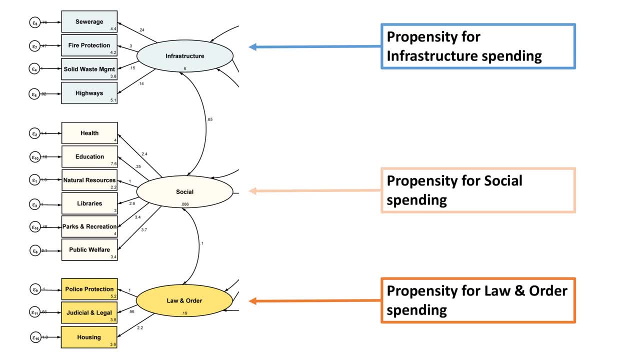 hopefully county health planners some indication of what matters the most. I'll just point out that in my county, Baltimore County, the county executive has asked the public to go on a website and actually go and use a SurveyMonkey, to use these exact same buckets and say what's the best way to save money. 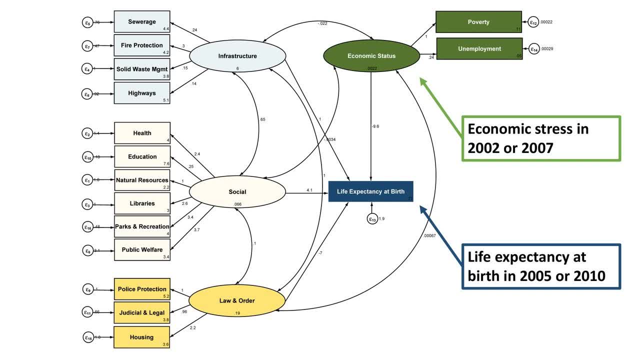 What's the best way to save money? What's the best way to save money, What they think should be cut and what should be increased for the county? The county executive board wants public input into what works. It's a democracy, and so that's nice, but I would hope that voters would like to see. 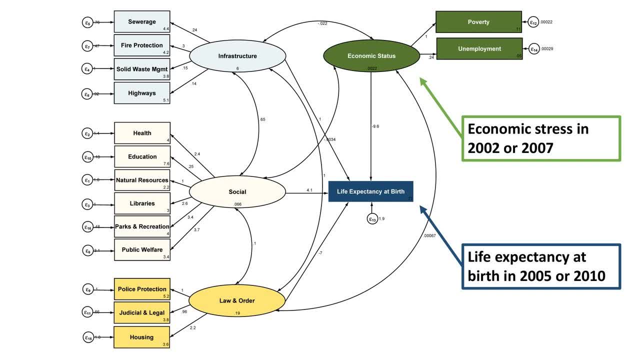 some research like this to see how the spending buckets affect their collective health, and that's what these results are intended to start a discussion for. So let me just close up Next slide. So here's a slide. So what we're finding and, best section, we found when we described these buckets of public. spending. we find that most of what was counted as public health spending was actually not public health spending, and just these three areas of clinical care- behavioral health and disabled services- count for almost half of public health spending. We see large variations across states and counties. 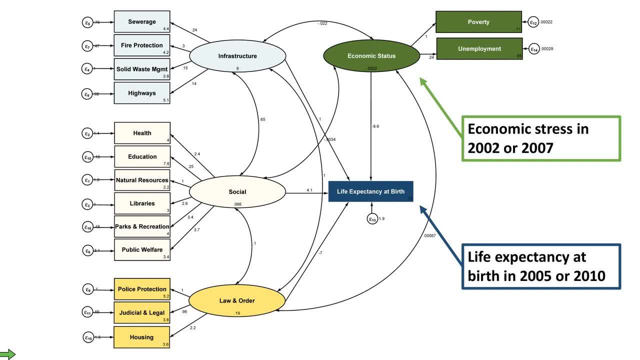 We see a flat trend in a lot of public spending on health, Despite epidemics in our county. we're seeing a lot of change In our country and despite what we know is a declining life expectancy, the states do not appear to be responding to this crisis with their spending. 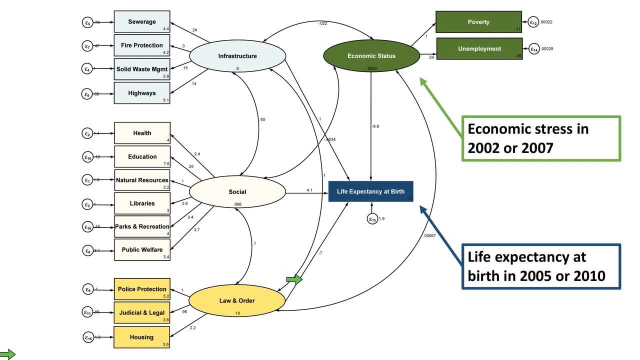 In terms of whether the spending can matter. our evidence is showing that yes to the states. If you think you don't matter, you're wrong. How you spend your money does affect life expectancy, and counting spending on social services is more beneficial than spending on infrastructure and counting spending on 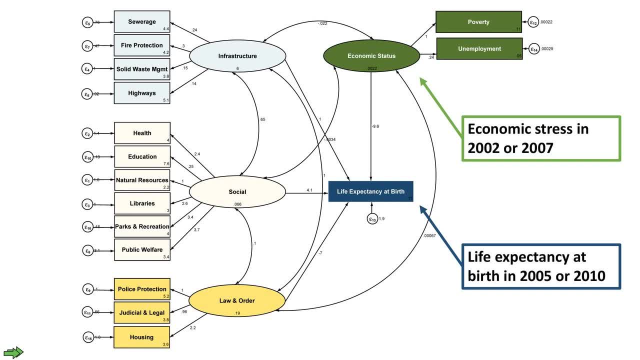 law and order is less beneficial to life expectancy as well. So we're seeing a lot of change. Dr Baruch, I'm going to turn it over to you. Thank you, Dr Baruch. Thank you, I'm going to turn it over to Dr Garvin and Dr Baruch. 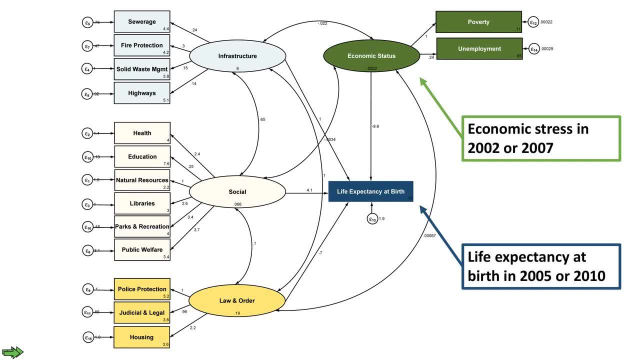 I'm going to turn it over to Dr Garvin and Dr Baruch. I'm going to turn it back and see if our results are. as of now, Let me go to the next slide. I'll turn it over to Marie for a discussion. 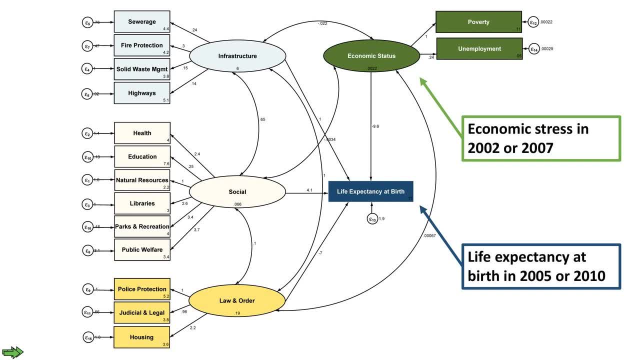 Great, Thank you, And thank you Dr Bashaw and Dr Resnick. I'm so pleased to be able to be a part of this webinar today. Let me just do a quick pause and say you guys are hearing me, right. 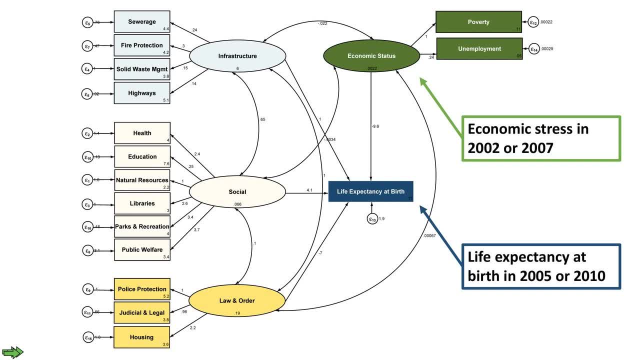 Yes, Okay, Thank you. This is such fascinating. research is so important to our field and we in the practice world are really excited to be seeing it and learning from it. as well as having academics learn from it, this kind of research is going to help influence thinking and 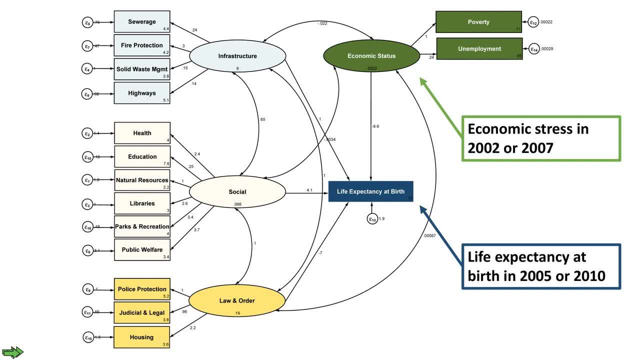 create in creating the body of literature. I think, as dr Bashar was just giving the example of it, can begin when it gets out into the public to help shift public perception and public sentiment and all of that together begins to influence policy. so I'm really looking forward to seeing more. 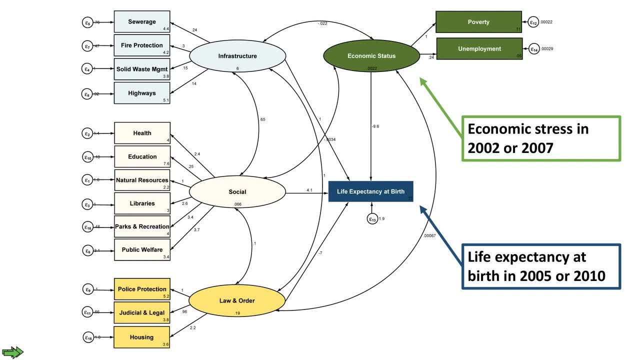 from this work and seeing where it goes next. so I'm just going to comment a little bit about what's going on in Washington and then try to lose plenty of time for questions for all. as dr Resnick was mentioning at the beginning, this work that's just been presented is such a beautiful example of kind of kind. 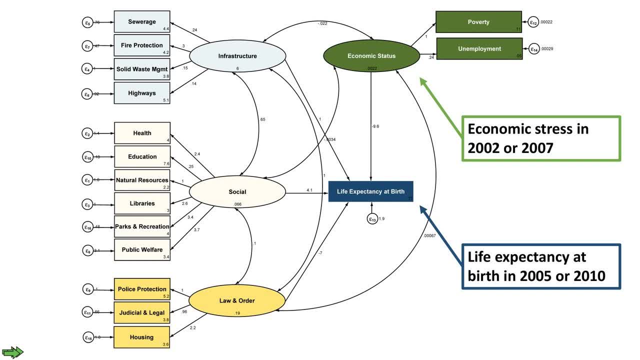 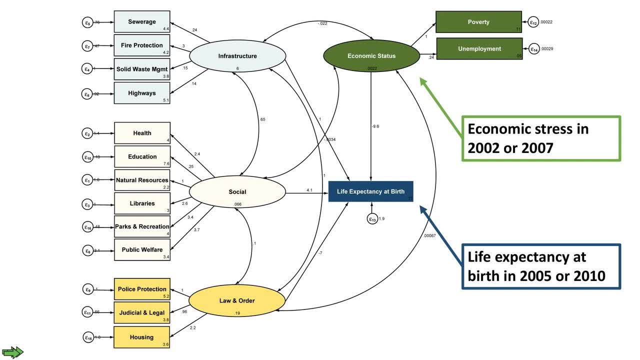 begin to dig deeper and ask more questions and get learnings from that. in Washington State, I'd say, we're at the micro level. we are working from the ground up. we also have data that is imperfect but that we can use and have our learning, so I'm just going to tell you a little bit about that in. 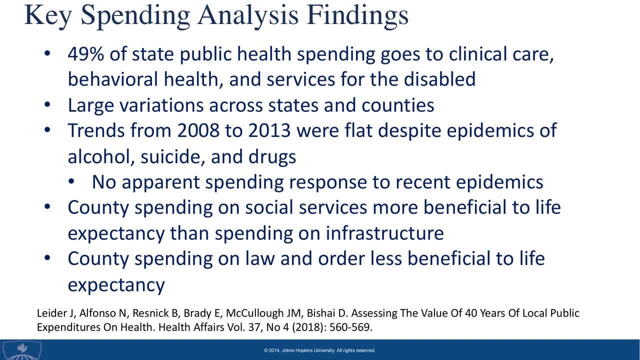 Washington State we have 35. I'm going to use the term County Health Departments, even though we use different versions of the name here- and we are blessed in that. for more than 20 years, we have been able to collect financial data from the 35 on how public health 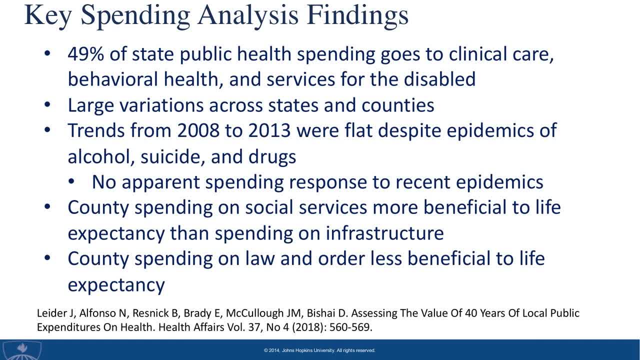 money is spent. this system is called bars. it's the budgeting and accounting and reporting system, because I'm afraid I'll probably fall into using that acronym. from that we can tell what categories of the money is spent on, similar to the categories you saw on an earlier side. 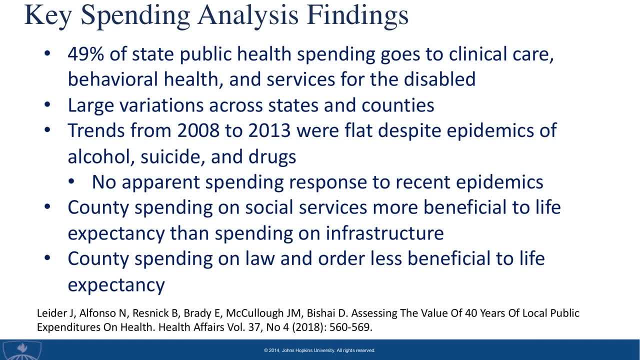 point public health categories- we can also tell the money came from, whether it was federal, state money, local money or from fees, So this has been a really useful resource. We're also really grateful to the University of Washington and the Northwest Center for 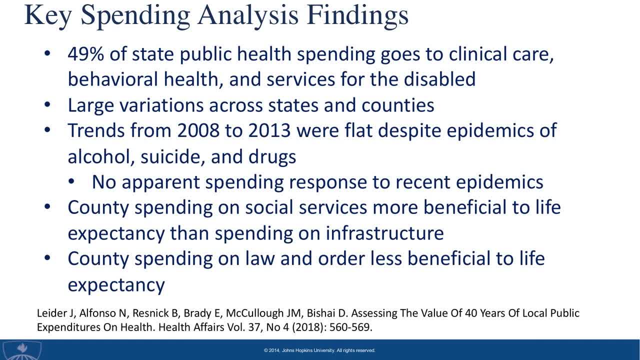 Public Health Practice, who has been putting years and years' worth of that data into the Public Health Activities and Services database called FAST, to help begin to analyze that. That has also provided, I think, a great stepping stone to the national efforts being led by. 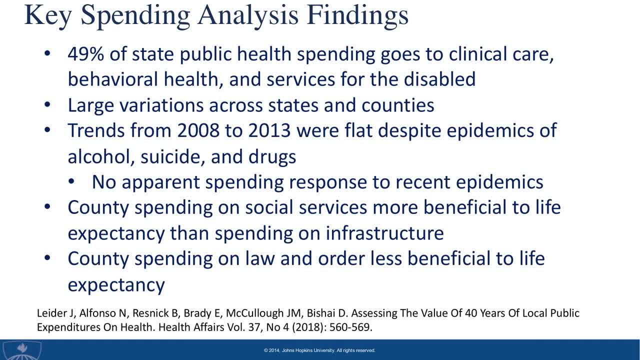 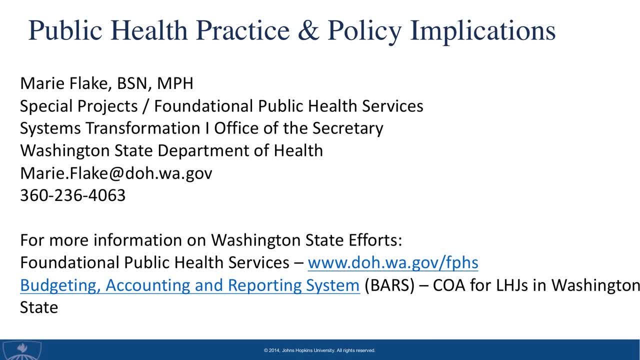 the University of Washington on a national chart of accounts to kind of get a little closer to that apples-to-apples work that was mentioned earlier in the presentation. I think this will create a nice linkage between local financial data and then the SHED work. 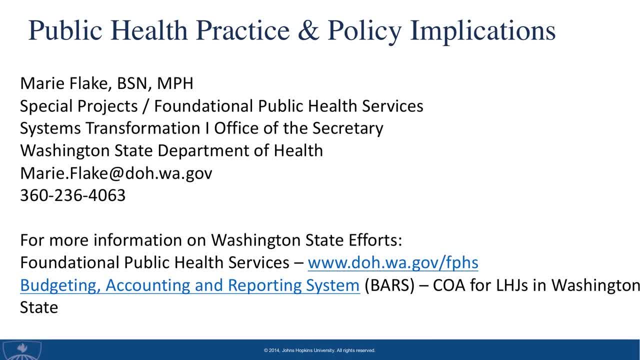 the state health financing system that folks here are talking about. In Washington we also have a state health department, and so when we traditionally have thought about a governmental public health system, we started by thinking about the county health departments and the state health department and can look at how money is spent across those. 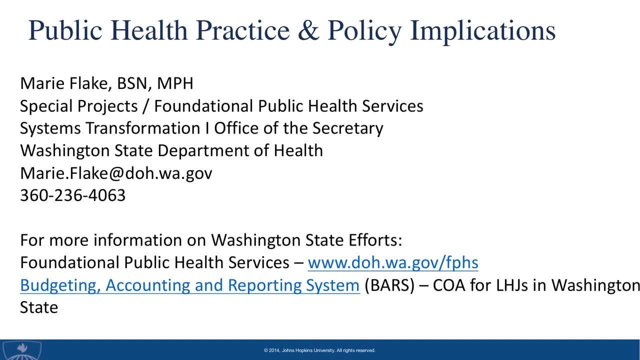 In Washington. there are also at least three other large and key state agencies that contribute to health, and that is the Health Care Authority, which is the Medicaid agency, also has other public insurance programs there. We have a state agency for social and health services and then a state agency for ecology. 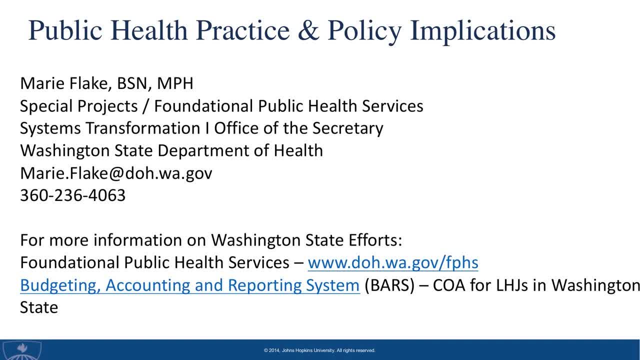 And so I. my perception is that probably data from all of these state agencies go into the census data that you've just heard described. so I'm grateful that researchers are beginning to tease apart that census data and try to find the public health content there. 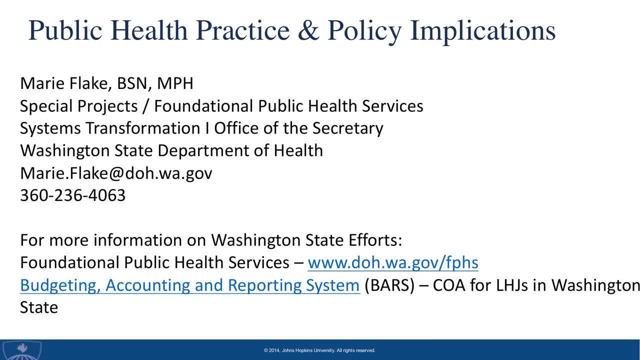 When we look at the data that we have here in Washington in the BARS and in our state budget, we can begin to see, like I said, how the money is spent in different parts of public health. like a slide you saw earlier, but we definitely have more to learn about. 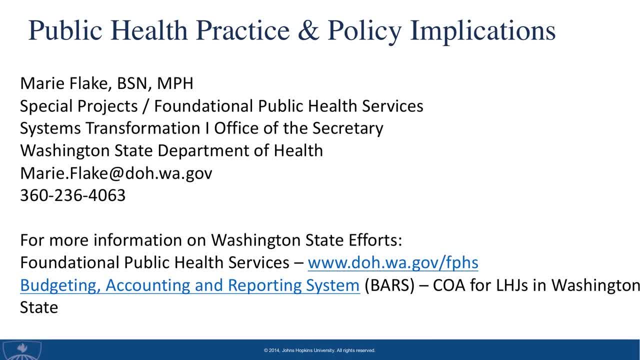 this census data. That is, that is going to this national level and maybe we can all do some learning together on that. I want to talk just a minute about the foundational public health services work we are doing, which is a small piece of the funding issue- kind of another angle on funding than what. 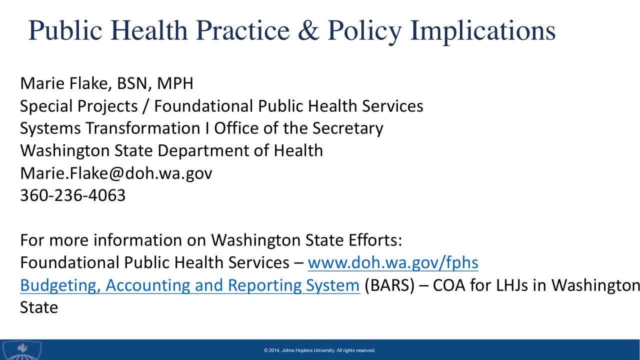 was presented here, but it has very related. We've been working to try to fix a problem that we identified as a lack of core funding for public health. Rather than funding the issue of the day and the current crisis of the day, we've been 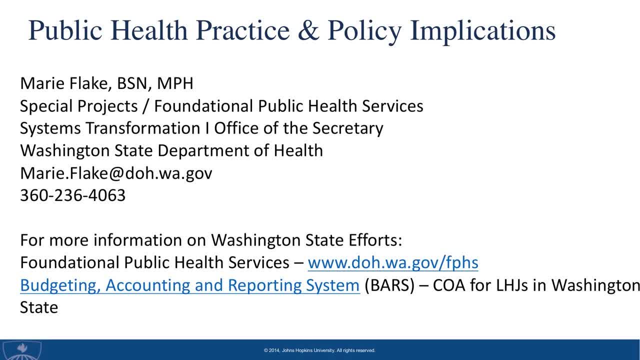 working to try to fix that. We saw that we often rely on federal grant money or kind of ad hoc funding for rising issues like that, but what we identified is that there wasn't any core funding really holding the system together, enabling the governmental public health system to look. 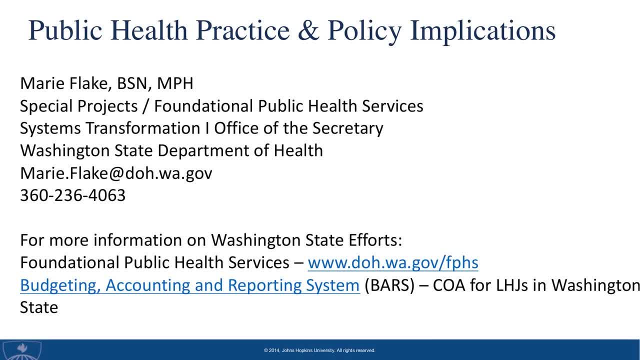 at the data and even collect and bring the data, such as we looked at earlier in this presentation, We had a broken and irrational and inequitable funding system in Washington state and that we need to monitor. We need to modernize how we do our work. 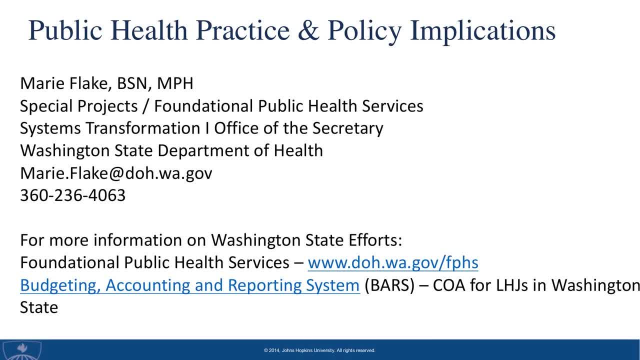 With that in mind, we set about defining the core activities of the governmental public health system. We took a very narrow focus because we thought we needed to again try to define the apples so that we could begin to compare apples and things like that. 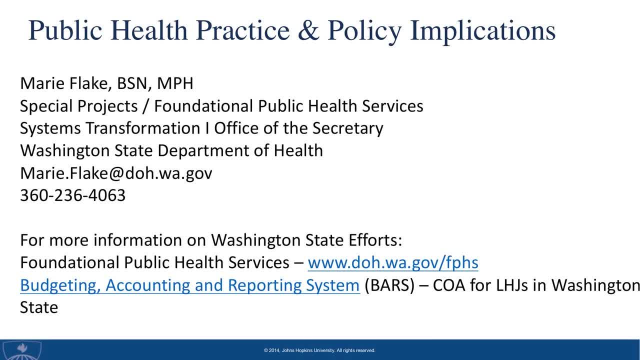 We defined these services. We defined what the governmental public health system consists of In Washington. we defined that as the state health department, the state board of health, the county health department and the 29 tribal governments and the urban Indian health programs that help serve them. 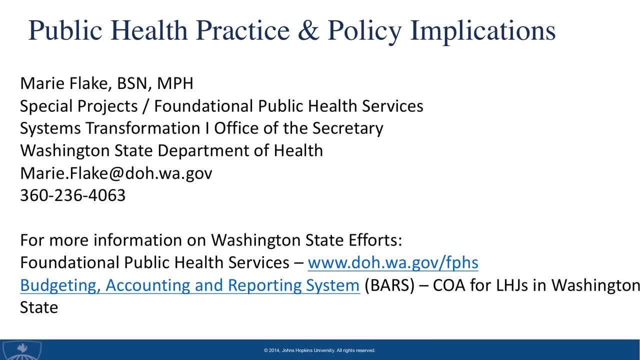 With that we defined this subset of services that the governmental health system provides that are core and that the government is the primary provider of everywhere. That is a smaller, more tightly defined list than what you saw on that earlier slide of public health codes, but it is kind of the work we're doing right now and the approach. 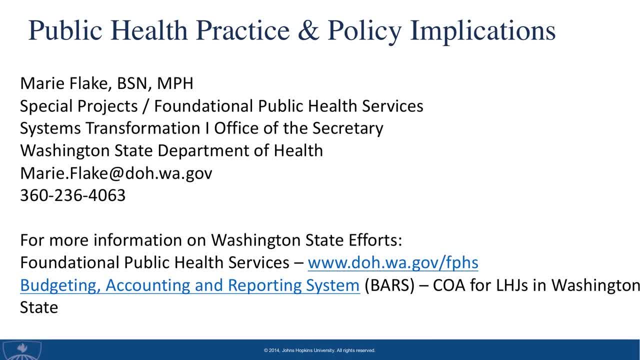 We're taking it step by step, Thank you. We're seeking state funding, state support for those foundational activities. Then local funding could be directed to local priorities, Kind of like Dr Bishara was describing- I think the term I would put on that sounds. 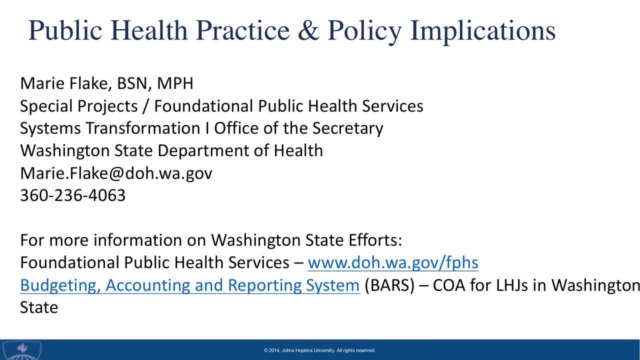 like a participatory budgeting exercise about how would citizens direct their local government to invest money. We could get to that point better, we believe, if we have a foundation of funding to work to make sure that the key activities of the governmental public health system. 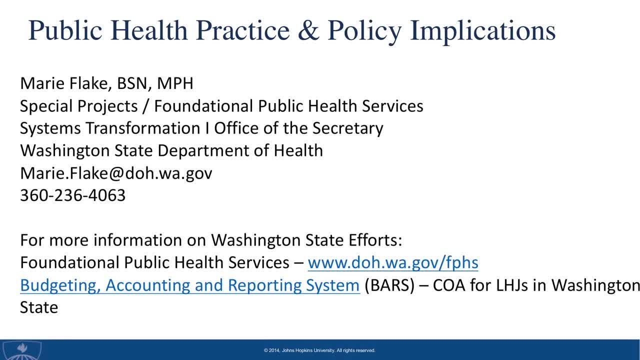 which are largely around data planning and coordination of partners, being that community health strategist kind of role would better enable both local government and then state and government who want when we want, to make additional investments in the issue of the day and the current problem with that we are. 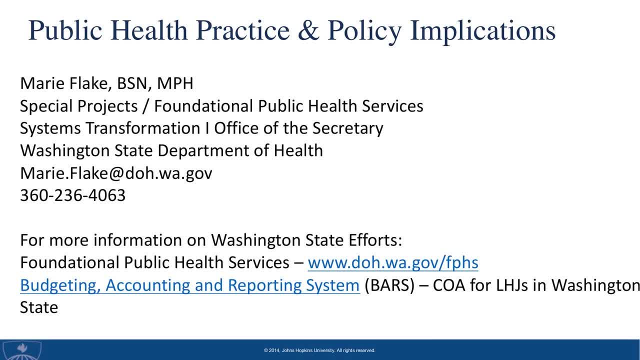 doing an accountability system so we can track the funds. part of that work is to update our bars coding, which looks a lot like the slide you saw earlier, but try to also add codes that tease apart those core services of government, separate from other public health services, so we can really track if we are building this. 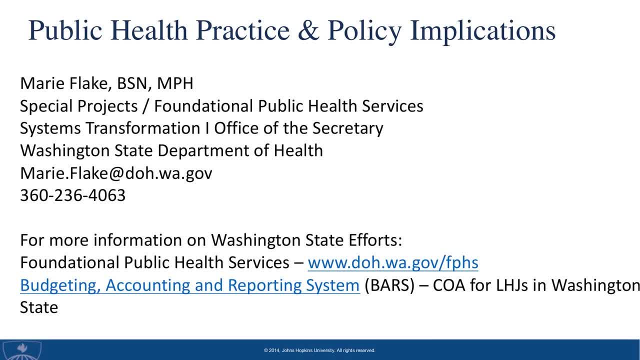 foundation. I think I'm going to pause right there and stop there and leave it open for questions, because we want to have ample time. I just want to close to say it's like again, very exciting research, again. I think, as you know, we've got a lot of work ahead of us and we're going to have a lot of 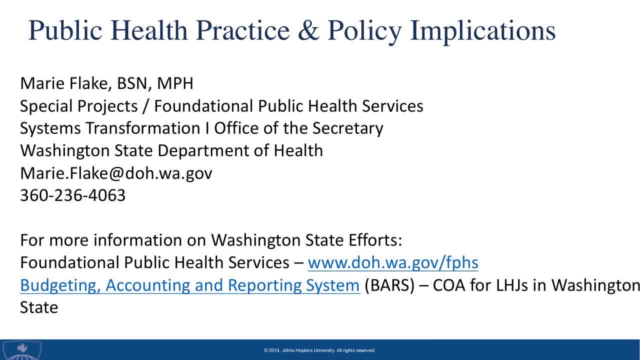 more research is needed. it would be great to learn more about how economic downturns and the fact that all this government money comes from the people, how that all plays together and competing priorities on governments and how that gets weighed with this propensity or prioritizing of where to. 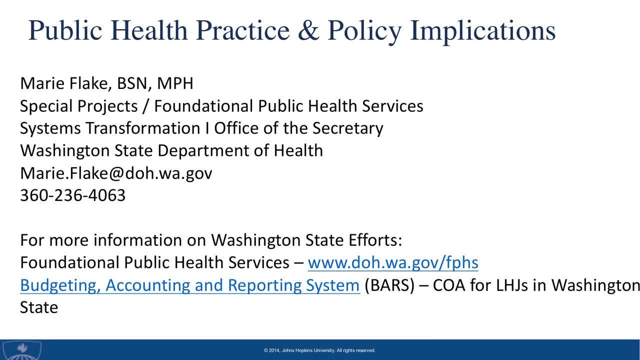 invest. so I'll end right there for now and thank you, guys. and chance to participate. great, this is Shauna. again, I want to thank all three of our presenters for reporting on this interesting subject and go ahead and get us started with answering some of the questions that have come in again. please feel free to type them in your 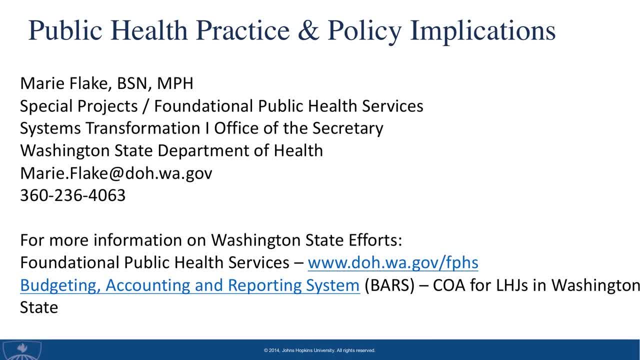 lower left-hand portion. as we begin discussing them now, the first question came in is: why is behavioral health not considered public health? maybe this is in reference to something that you had mentioned, dr Resnick, in the beginning of the presentation, right so when I was categorizing what is using that, 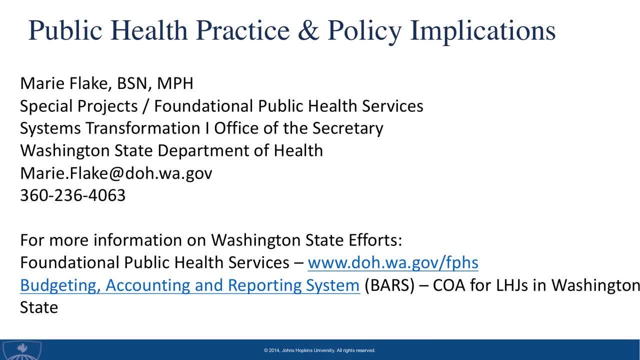 foundational services framework, what is public, what is considered public health versus other health or services? so behavioral health is clearly health and services, but it's more geared at individuals. so, say, a common thing now is substance abuse counseling or treatment, so that is directed at an individual, whereas in the 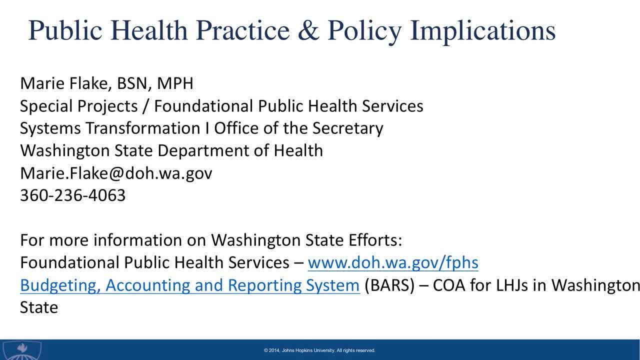 foundational public health services. you're thinking about population level activities. so, for example, if you were doing a drug prevention program and you're going to public schools, schools and communities and doing education and outreach, that would be more population level. But behavioral health itself is more of an individual service. So that's in the 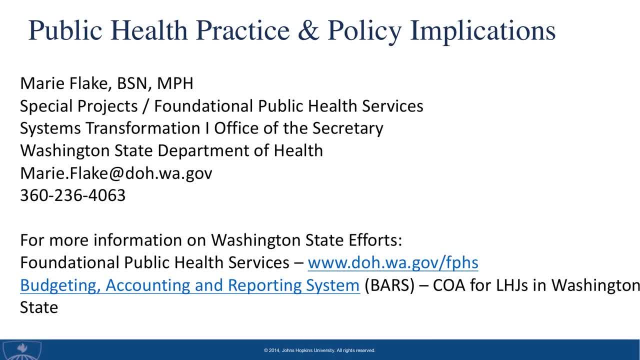 model. That's why it's categorized differently. Okay, great. The next question. I think maybe Dr Bishai was discussing the model And this particular person would like to know if it would look different if housing was part of the social spending rather than the law and order section. 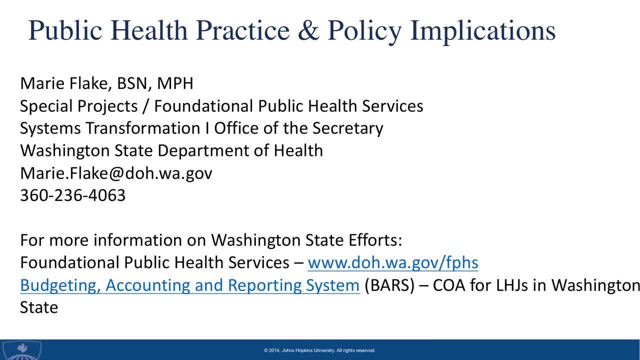 Yeah, this is David Bishai. Absolutely good suggestion and good question. So, as I said, we have been really working on what indicators should go into what category And we spent time asking the data to just say where does each you know spending category want to? 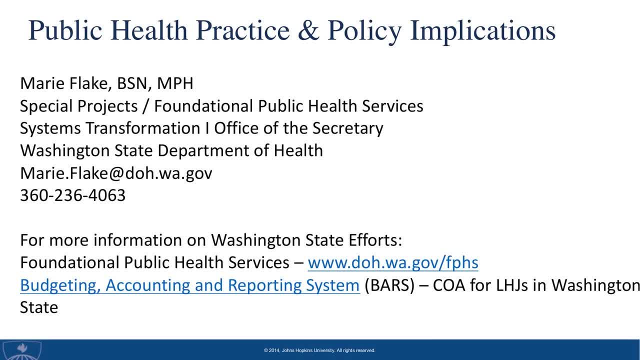 naturally go- Yes, naturally affiliate. and when we did that, we couldn't make any sense of it. The data really doesn't want to naturally affiliate. and when we find out why, it's really because I don't think they have a natural way of making data correlate. 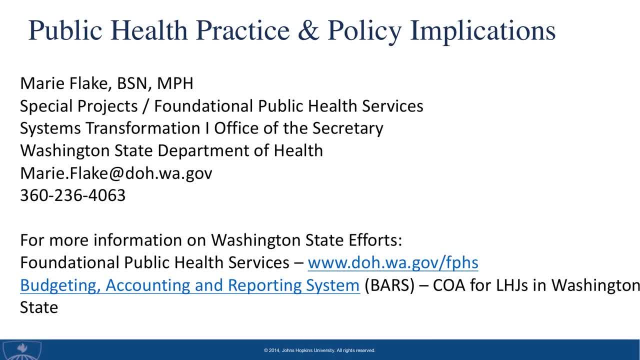 So back to your idea. maybe you can use the chat box to say more about where you think that housing might end up. We thought that a lot of the housing spending goes into public housing as well as home inspections, permits and building, and would relate to where we thought some of the regulatory 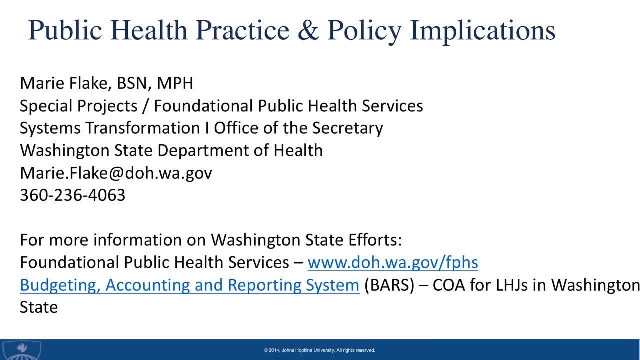 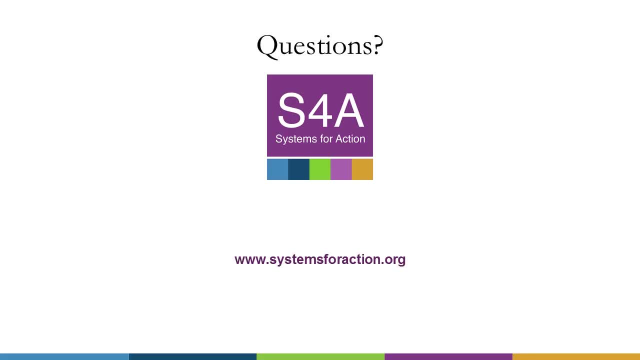 operations would be giving people permission, but if a given county is less on the regulatory of who gets permission And perhaps in an urban setting, actually using their money on giving rent for low-income housing, it would be much more like a social or an infrastructure. 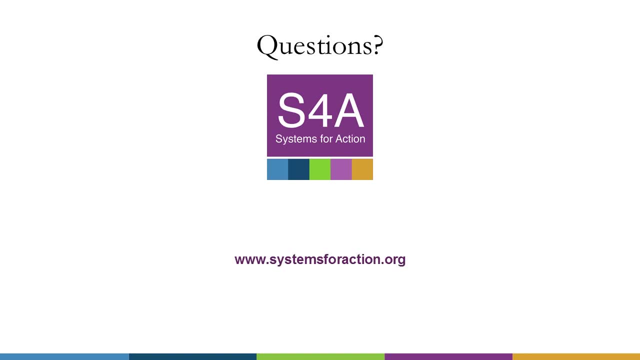 So, thanks to your suggestion, we can go back to this model and move housing out of its current area and into another area and see what that does to our goodness of fit and to our model and see if our results still hold, and I think that's a great suggestion. 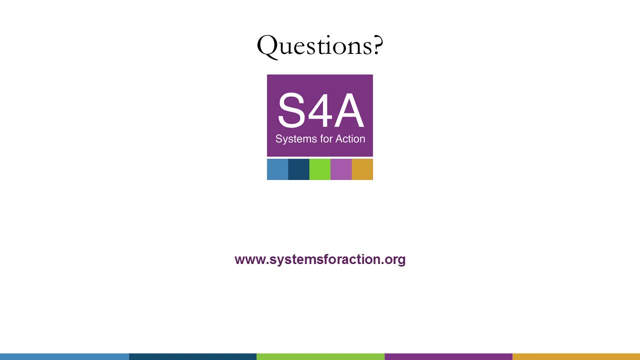 which is why we do these seminars. All right, Excellent, Okay, This one looks like it's for our commentary speaker, Ms Flake. This person would like to know how Washington determined the foundational public health services and how did you get an agreement from local and tribal public health entities? 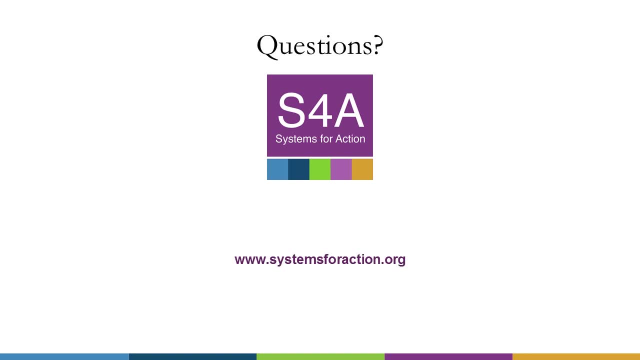 on what those services are. Okay, great, Thank you for the question. Let me start by saying the tribes have joined more recently And they are currently in their own process- that is tribally led and tribally driven, to define foundational public health services relevant to them. so stay tuned more on that. 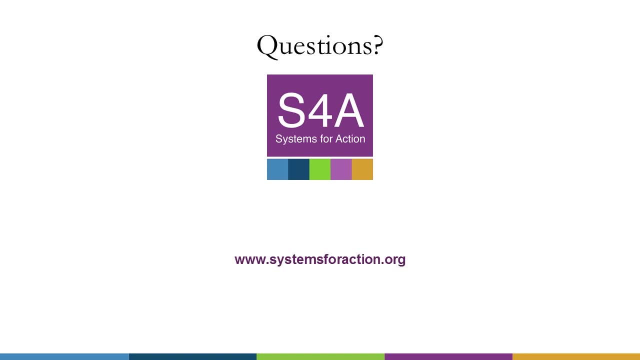 later. As far as state and local traditional public health partners, this work sprang out of a long history of joint state, local statewide committees working on various projects And in 2011, the latest iteration of a public health partnership was established in Washington. 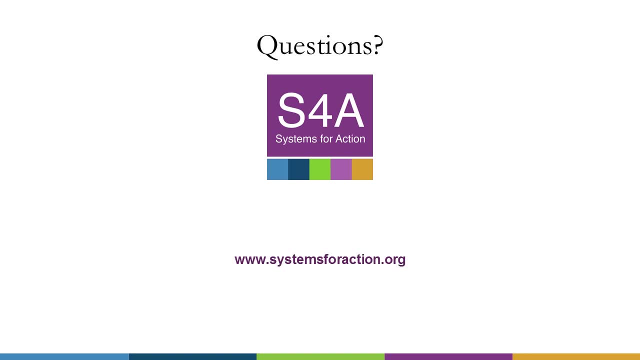 DC, And it's a great project. It's a great project, Thank you, And we've had an excellent partnership with the National Public Health Finance Committee that was formed, that was co-chaired by a state person and a local person, and that. 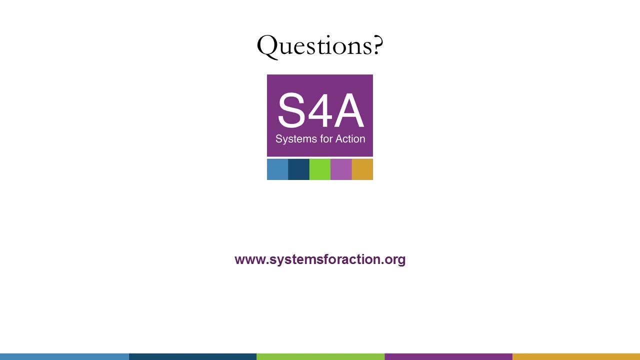 is the group that invented the idea. that is like, wow, if we're going to ask for money, maybe we better define what it is people are going to buy. And that's kind of the origins of this foundational public health services idea. And so criteria: the committees together invented criteria that largely in a nutshell: 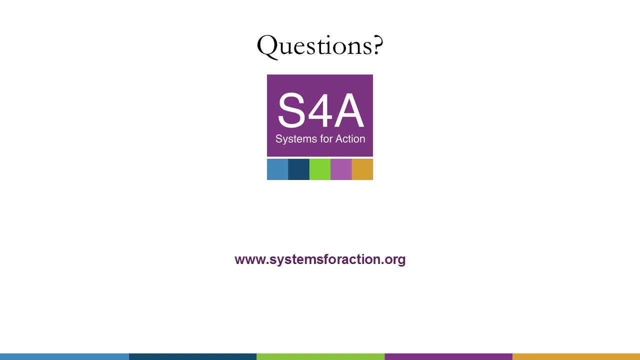 were. let's identify the services that only government provides, and thus government should fund them. they need to be provided everywhere by government services that are population-based, and then let's pay attention to what is mandated. that itself would not be a defining characteristic, but you know things that? 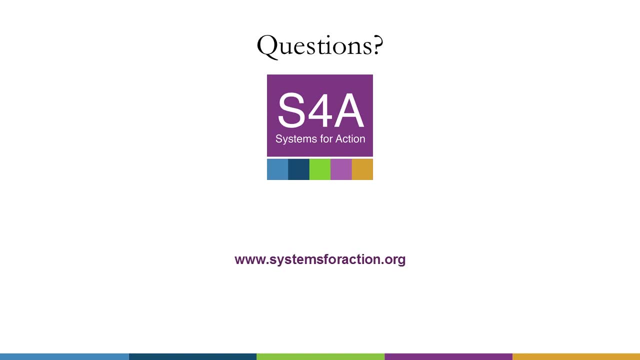 are mandated. we either need to deal with or change the laws. things that aren't mandated might have a little less traction but still could be foundational. so that was the criteria and then the group went through years of many dialogues and conversations and debates about: is family planning, for example? is 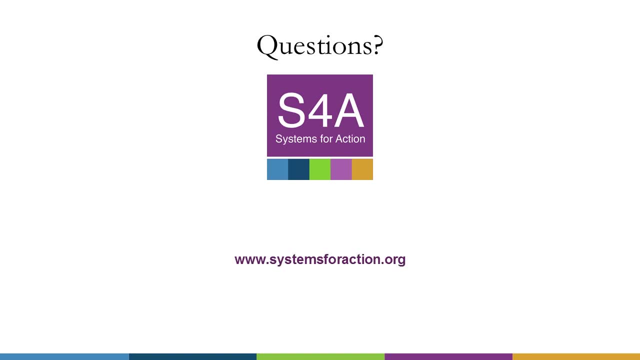 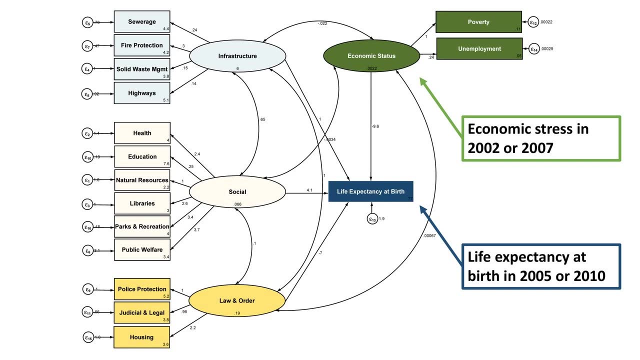 that a foundational service of government? and the conclusion was no, because, while it is an additional and very important service of public health- greater, broader field of public health and, in some cases, government- a county health department might be the provider of it. government- in our definition, state-local, not federal, but state-local- is not the sole provider of this across. 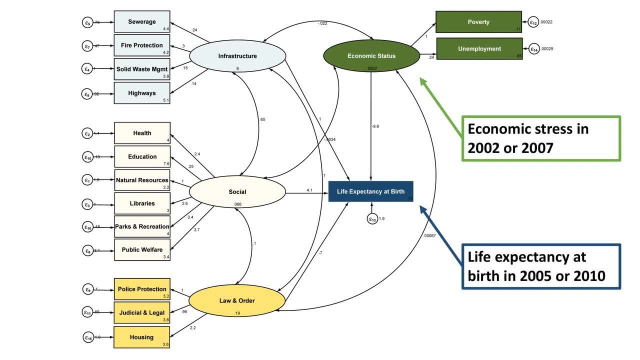 our state-local system, but it is the sole provider of this. across our state-local state we have hospitals, we have clinics, we have community health centers, lots of providers who do this work. so that's it's been a dialogue all along and it's been the ongoing dialogue to this day, as we continue to think about when and how. 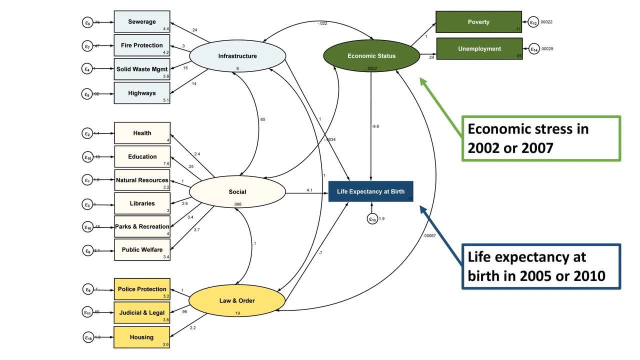 we update these definitions. all right, excellent, okay, I'll just go ahead and take us straight into the next question. it looks like it's: how might unmeasured or imperfectly measured need and demand for services effect results, particularly if intergovernmental funding formulas are partly need-based? so this is, David, let me try to think about that, that question. 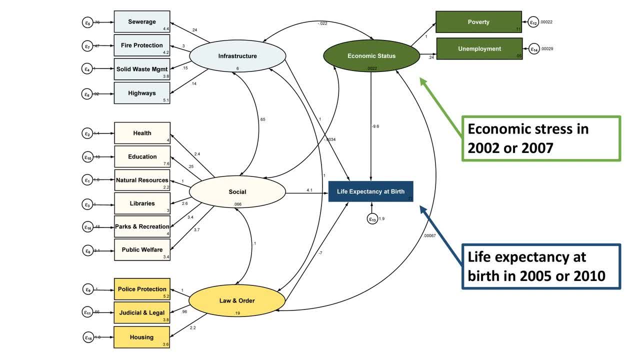 and what I thought our way of work was that that a rising death rate in a in a state was an indicator of need and I think that was responsive to that idea. one could take that idea also with a rising death rate in a county and and show that in 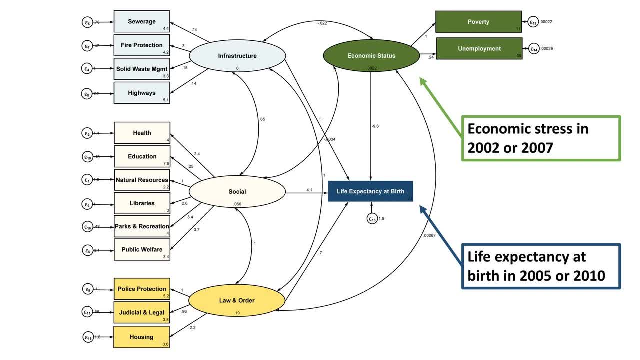 some of the work that we published in health affairs, we began to look at a ranking of different counties into having declining economic fortunes as well as declining health. that's a great question. I think it's critical that the look away is that you then have to understand where they compared the 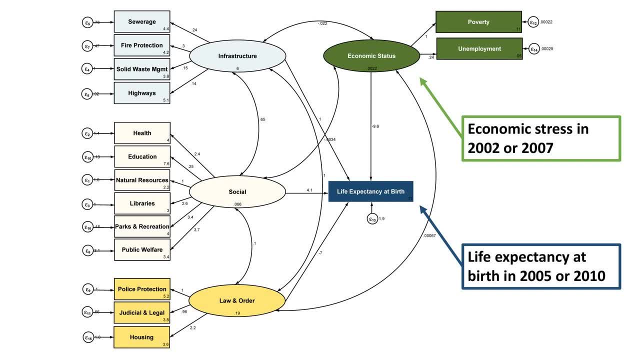 full population range, if you were to find an community agent, and then that was the ideal model. but, that being said, we don't. Are they going tolingen the reality in America that the sickest counties, with the lowest life expectancies, are not coming out of their slump? They're not bouncing. 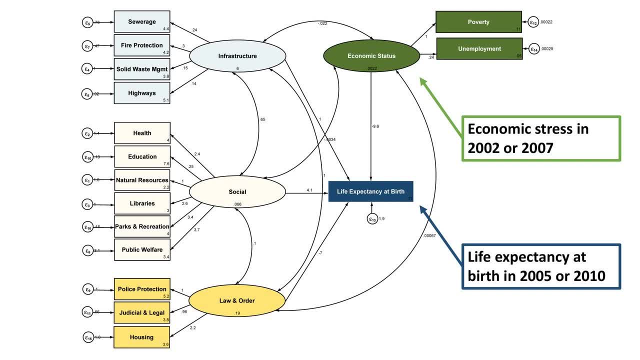 back: The sicker and poorer you are the sicker and poorer you get, and the richer and healthier you are, the richer and healthier you get, And I'm sensitive to the great idea of having that be some indicator of need In a system where you have to finance your own county health budget with your own property taxes and you don't get help from the richer counties. what our current research shows is there's no correction that there will be a rising disparity between rich and healthy and poor and sick, And it literally would require a state. 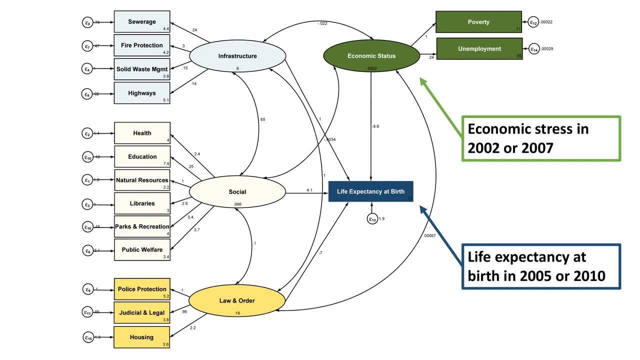 legislature to do intergovernmental transfers to correct it. I'm glad that there's interest in in this audience in that type of work. I think it's really important. I think it's really important. I think it's really important legislative reform, because in a democracy the haves don't always want to. 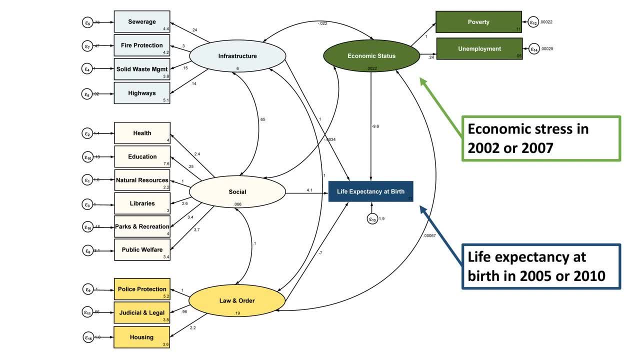 share with the have-nots. There's not a sense of solidarity and it requires research to show the problem for the haves of living in a county with the have-nots. Certainly a measles epidemic ought to be a wake-up call that if you let go of your neighboring county the measles will. 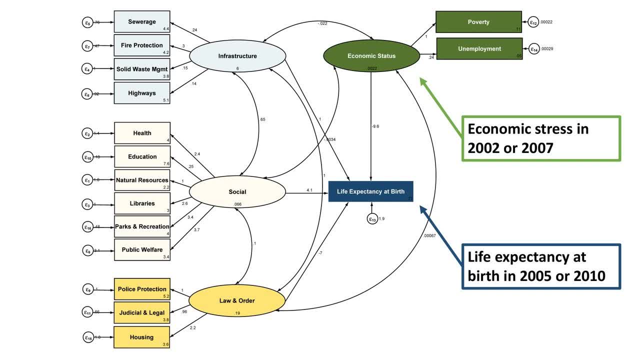 cross the county border And I really think the research community can can contribute to that narrative. This is Marie. I'd like to add to that, if I may, on a conceptual level. I think what Dr Bichaud just described. it was so eloquent and it's a part of what's. 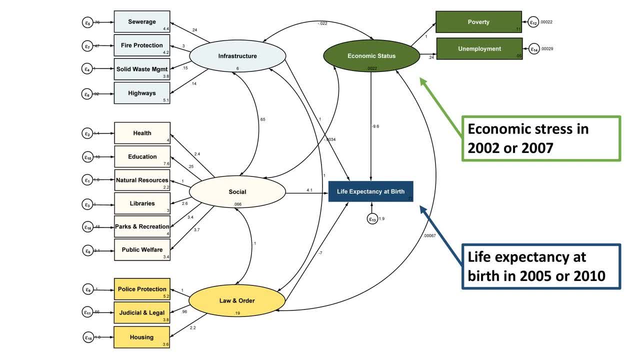 underlying the work we're doing in Washington. Again, while we are focused on a small piece of the puzzle here- the foundational services. we haven't yet gotten to those additional important services and the actual need in that way. But what's, I think, really? 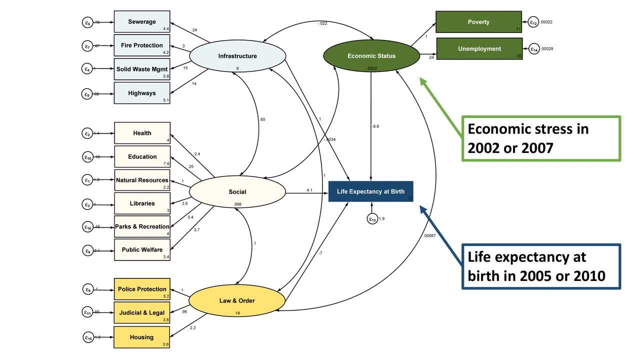 different for us this time, as we are doing this approach this time around, is we're really trying to stick together and hold the line on. we are trying to fund a system, not 35 county health departments and the State Health Department, because that always backs us into the corner of what Dr Bichaud just 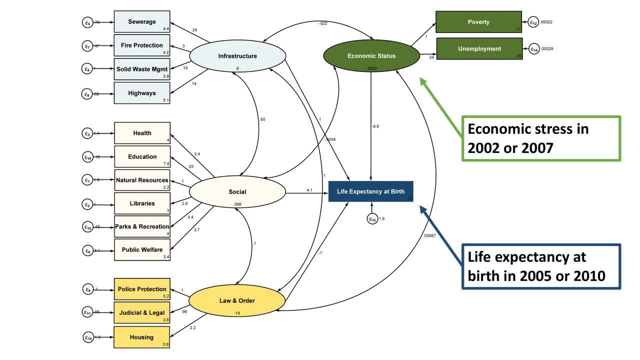 described rich and poor, and then you fund your own And it's harder to share when the lines are so clear that this is mine and that's yours, When we're really working hard and it is a challenge every day to take a systems approach and say if the people of Washington need. 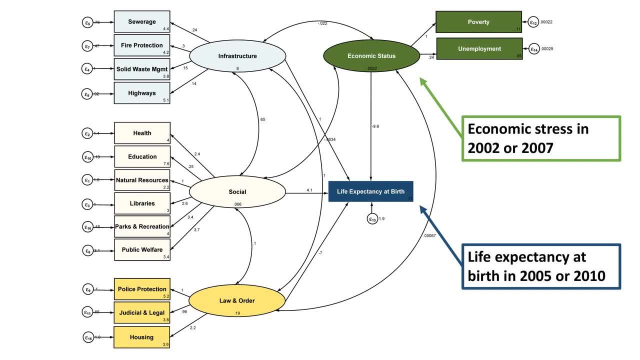 this service. you know how do we fund it, how much does it cost and how do we best get it delivered to them, working together, not working as you do that and I do this. so it's a subtle philosophical shift, but we are optimistic that it has some real promise for us. so, Marie, this is Beth. that's a really great point, and 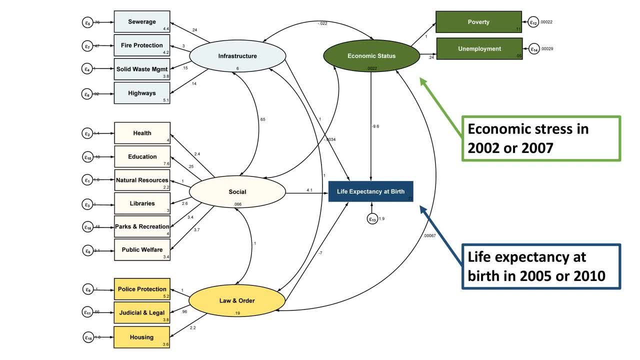 very admirable that Washington State is doing that and I think it's a great model. but I have a quick question for you and David, because I felt there was a little bit of a contradiction in things that you both said. so, Marie, you talked about having the infrastructure, because when a crisis hits, you know, then all the 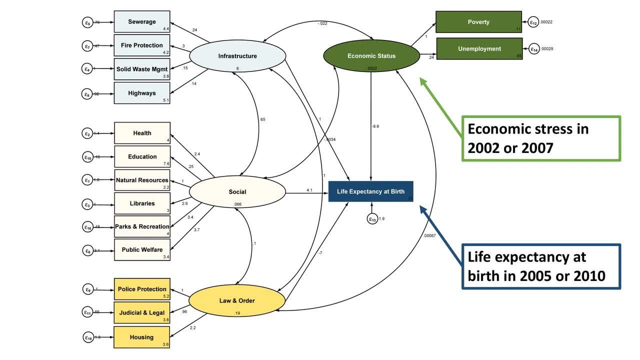 money shifts over to that and you have no money. but David talked about in his presentation that the spending has actually stayed flat and it doesn't change based on any kind of crisis. so I guess my question is: is that because we're in the middle of a crisis and we're in a crisis and we're in a crisis? 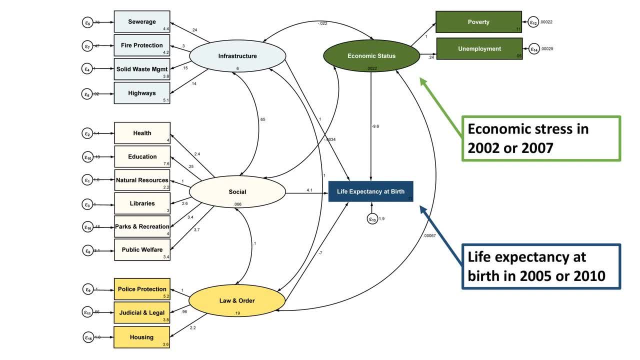 we're talking more about the non public health dollars, like the health services, like, say, behavioral health, or is there a shift? is the data we're looking at maybe not telling us the whole story? wondering if either of you have comment on that. yeah, this is David. um, I think that what Marie's talked about in Washington, which 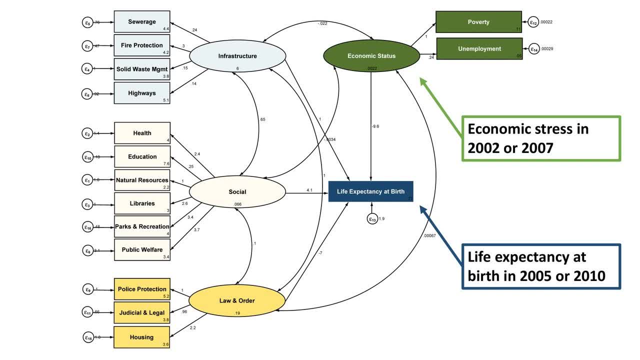 is the core funding. I see core public health funding related to a core public health mission of politics. this is a core public health mission of politics. this is a political act. to be a public health office requires getting a consensus that the people are having a health problem and they should spend. 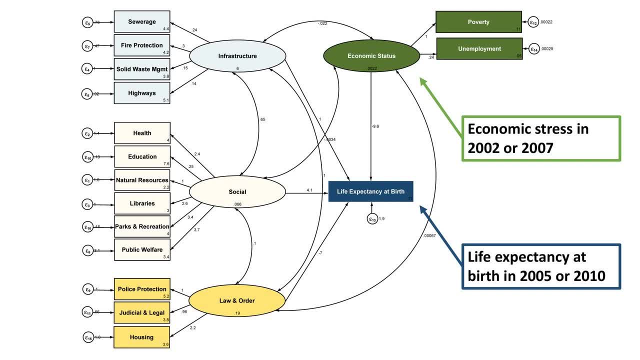 something on it, and you can't do that if all of your funding is tied to one disease. if you are there with family planning money, you're not supposed to do any politics, not let alone you're a public sector employee. but traditionally in the 150 year history of public health, the untied funding has been consciousness. 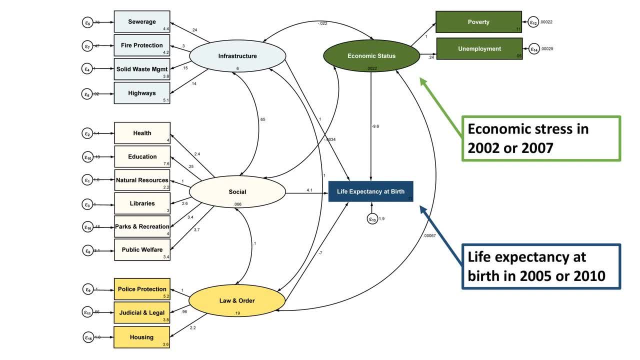 raising politically motivating work. and yes, I understand how it's hard to be good at politics when you're being paid by the public purse. there are legal reasons that you can't, but then, obviously, is what we have to do to inform people about what's killing them and to suggest there are things to do. 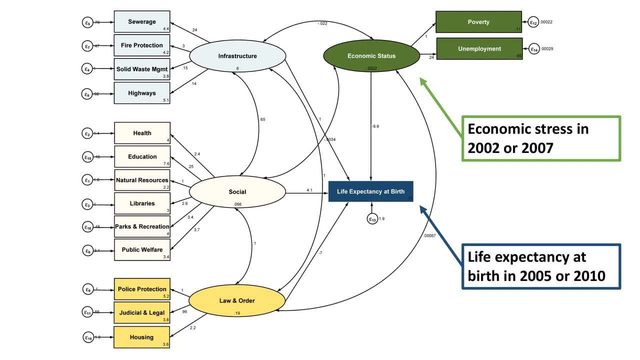 that is actually a political act and it's totally legal because they wake up, there's an epidemic. you can't do that. you can't do community organizing almost freely. but really, if we built it, that is true and frankly, people don't do it just as you see it. everybody else does and I think I see, othermentally, i agree. 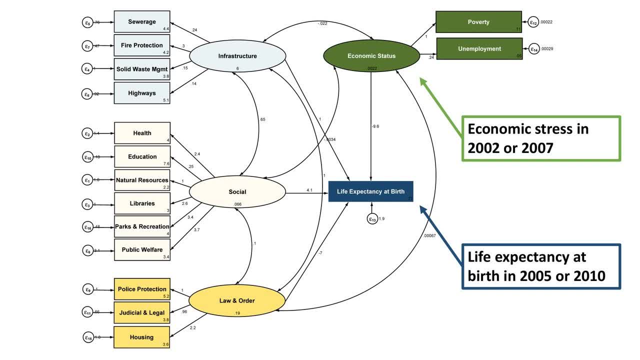 it's all your money tied, and the reason that the budgets aren't moving is political, and it's related to a lack of resources as well as a lack of ability. I think that the public health profession, the ones that we train as educators, just don't see their role as community organizers. 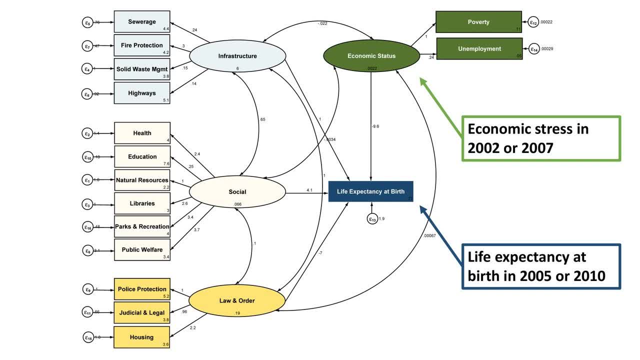 and political mobilizers. I think that was so well said, thank you. I think just to add small bit to that is that you know funding. I know that core and infrastructure isn't always exciting or sexy, it doesn't always sell because it's not the opioid epidemic. but the problem is: is the opioid? 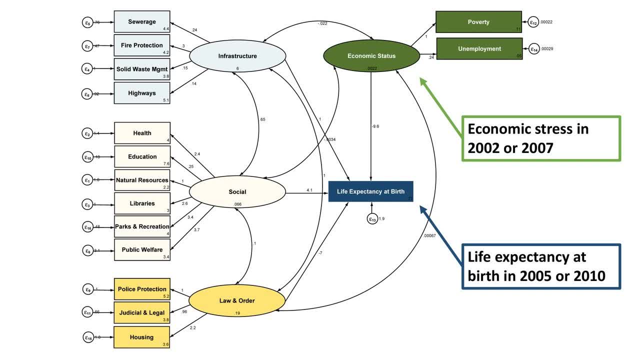 epidemic got so far down the road it's because we didn't have core, we didn't have the data, we didn't have the staff to look at the data, we didn't raise the flag saying hello public. we have a problem here. until it was so late and so 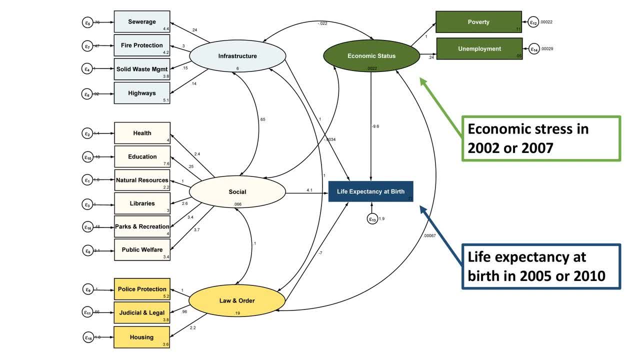 far down the road. so that's where the core is so important. it is exactly as Dr Bichotte just said: bringing the information to the community as a whole, both policymakers and the public, so that people can get, or get energized around. wow, we have a growing problem here. let's redirect, or. 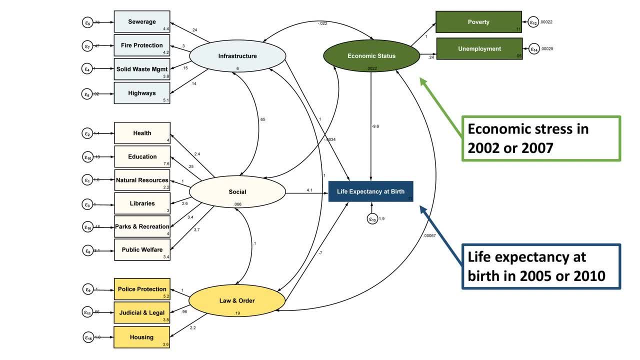 let's prioritize or let's change our propensity for funding to make sure that these issues get taken care of. so it's funding data, real-time data, funding, that convening of community partners, because government and public health agencies are not the only ones who work on this, these problems.